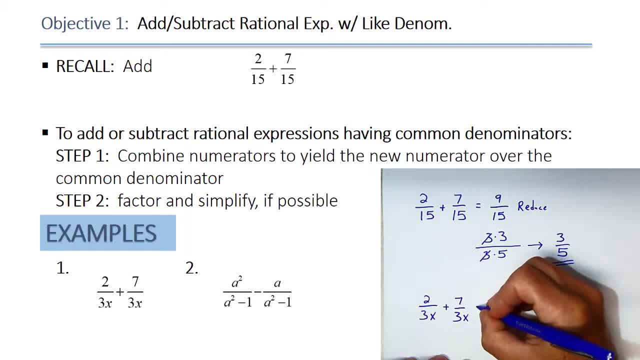 2 over 3x plus 7 over 3x. well, that's pretty easy. We can add those up and we get 9 over 3x. But can we reduce that? Well, we sure can. That 9 and the 3 both contain a factor of 3, so we can divide both by 3, and instead of 9 over 3x, 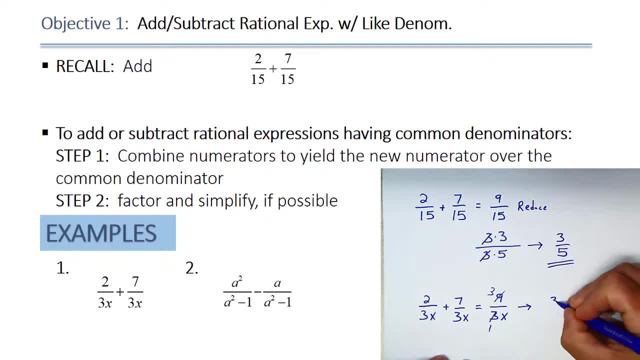 we have 3 over 1x, But of course we aren't going to write 1x, we're just going to write 3 over x, and we've got that addition completed. Okay, for our second example, we again have common denominators here of a squared minus 1, so we can combine the numerators. 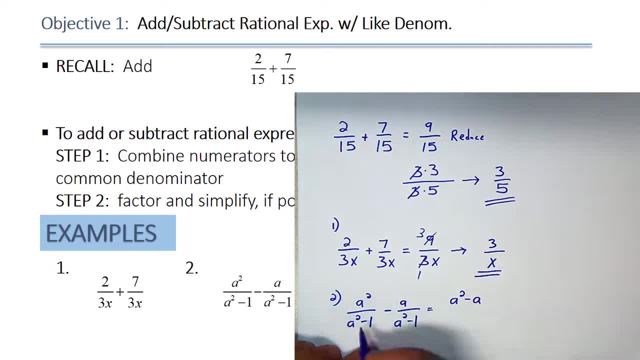 If we do that, we're going to get a squared minus a. those are not like terms, so we can't put them together: a squared minus a over a squared minus 1.. Now, here we go. Can we cancel those a squareds? 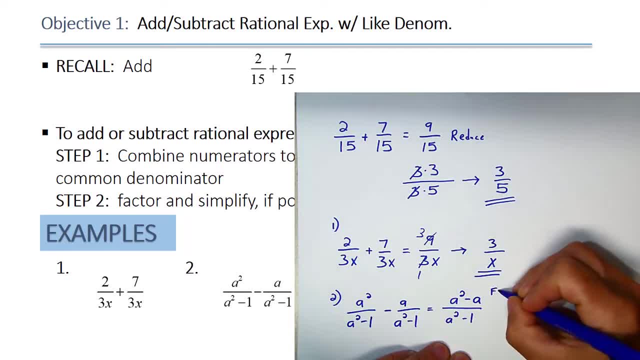 No, you're not going to fall for that. Those are terms. We need to factor everything and if we do that, this becomes on the top. we have a GCF of a That comes out and leaves us with a minus 1, and in the denominator that's a difference of squares. 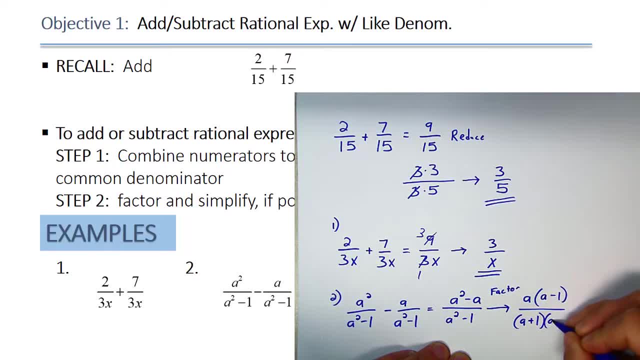 That means that it factors into a plus 1 and a minus 1, and now that we've factored everything, we can look for common factors. and, sure enough, we have a common factor of a minus 1, and that leaves our simplified fractional result of: 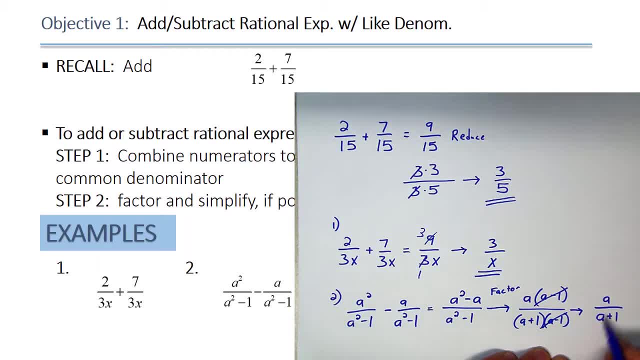 a squared minus a squared minus 1.. A over a plus 1, and of course those a's don't cancel That bottom left. a is a term, and so we've combined those two algebraic fractions. But of course, what if those denominators are not the same? Let's do a little refresher here. 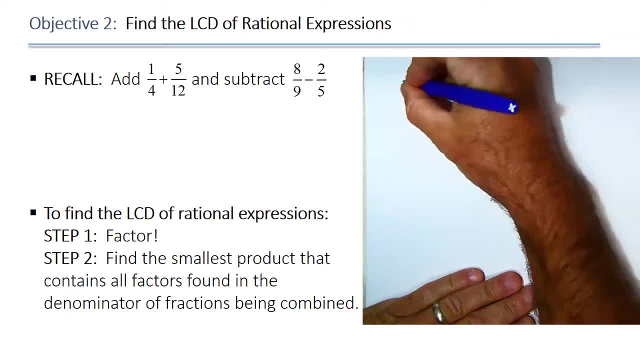 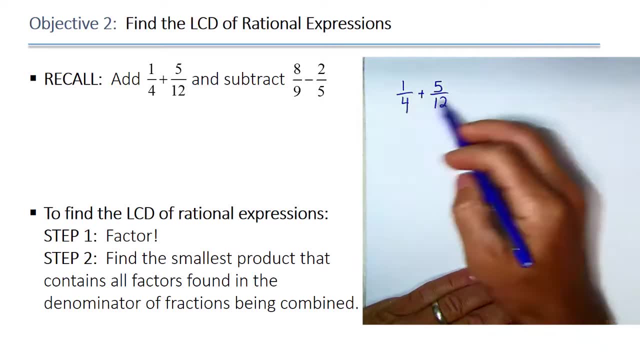 What if we want to add 1 fourth plus 5 twelfths? Now I trust that you could do a simple fraction problem like that, but let's look at what's actually going on here If we factor those two denominators. 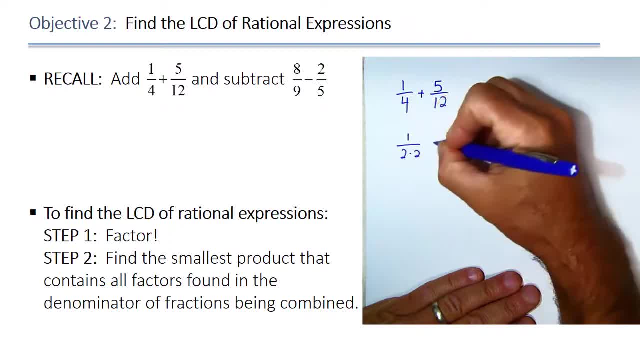 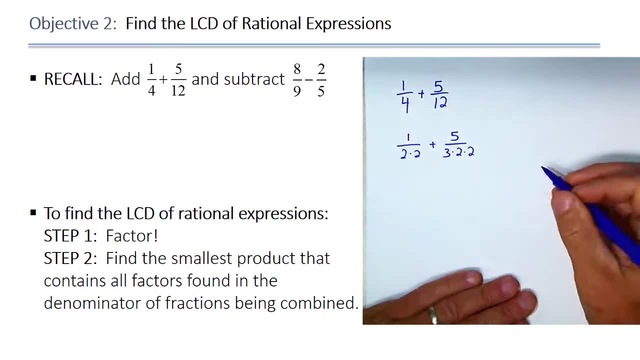 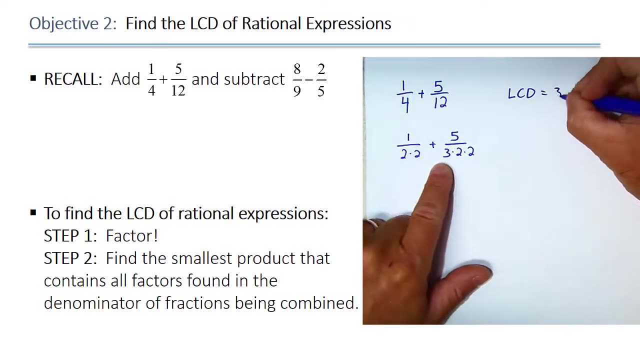 we would say that our first fraction is 1 over 2 times 2, and 5 over 12, that's 5 over 3 times 2 times 2.. So what's your common denominator going to be? Our LCD is, of course, 12,- we could tell that, but it's got to contain that 3, and it's got to contain 2 twice. 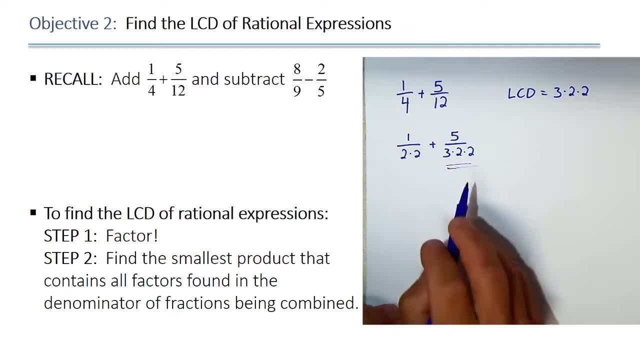 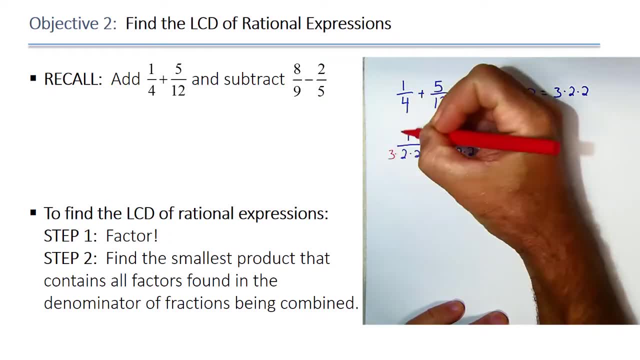 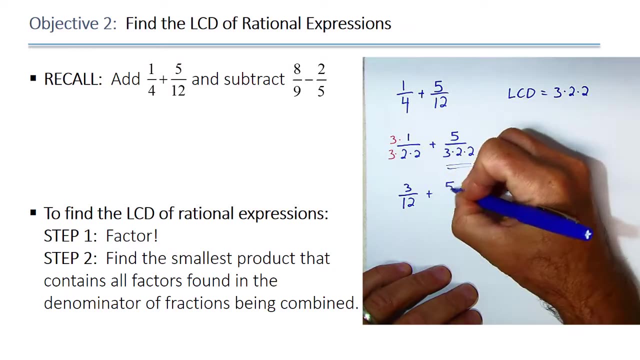 So that sort of tells you that this fraction on the right is ready to go and the fraction on the left, that's missing the 3, which is why, back here, to get a common denominator, we'd multiply it top and bottom by 3, and then of course, that becomes 3 over 12 plus 5 over 12.. 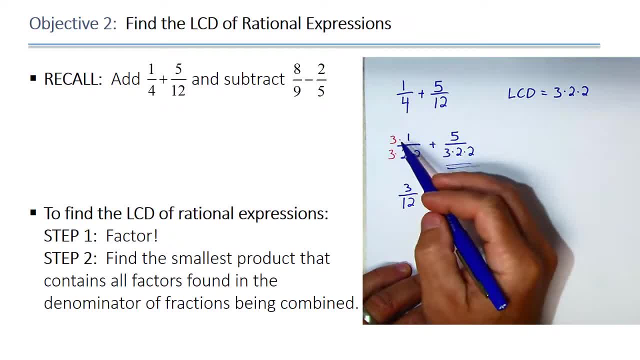 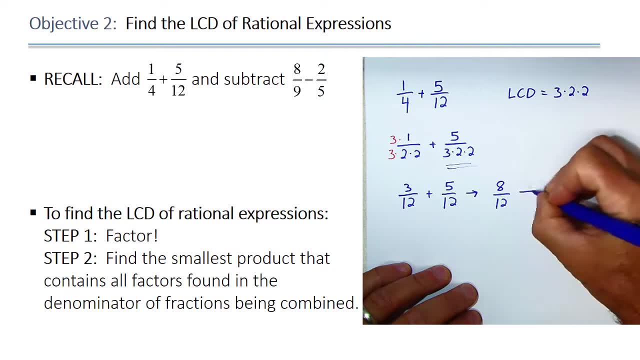 Now, that's a roundabout way of getting our result, but it's this: looking at the factors that we're going to need to do with algebraic fractions here in a minute That combines to give us 8 over 12, which reduces to become 2 over 3, and we've performed that addition. 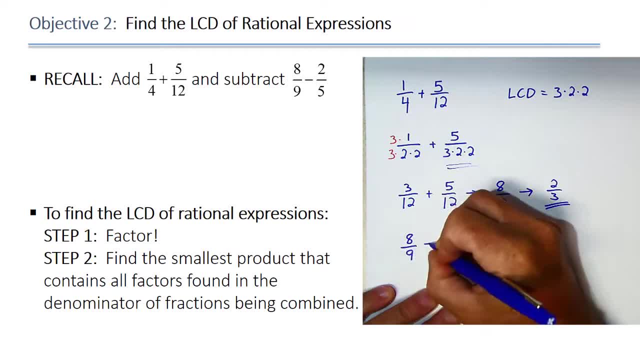 One more here. What about 8 over 9 minus 2 over 5?? Well, our common denominator there is going to have to have a 9 and a 5 in it, or a 3 and a 3 and a 5.. 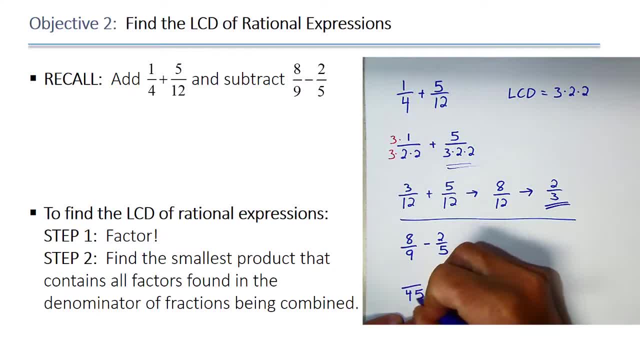 It's pretty clear that your common denominator there is going to be 45.. So what factor would we need for this fraction on the left? We would multiply both of those by 5, and that makes the fraction on the left 40 over 45.. 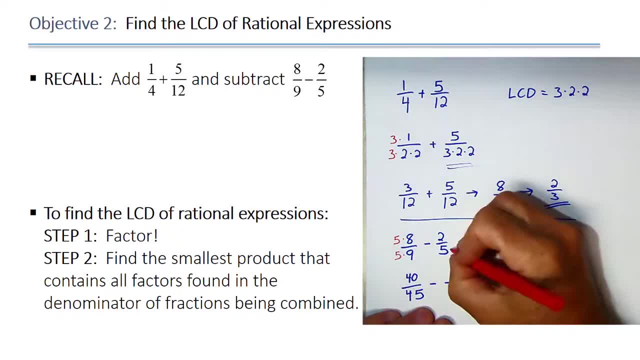 The fraction on the right has the 5, we're missing the 9, so we'd multiply in 9 on top and bottom there, and that un-reduces that fraction to become 18 over 45. Now that we have a common denominator, we can combine those 40 minus 18, that's 22 over 45, and we're done. 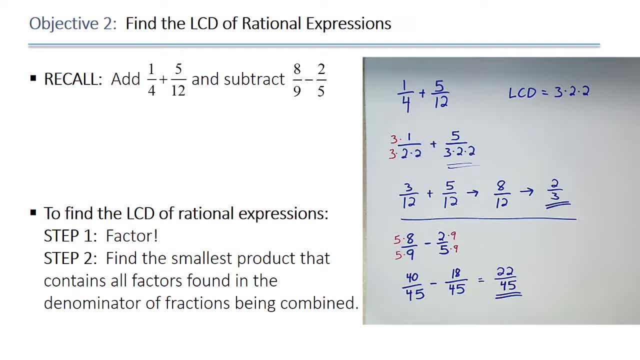 So the key there is: we want to factor if necessary and then find the smallest product that contains all those factors being combined together. Let's take a look at some algebraic examples. Okay, so let's combine 3 over x plus 4 over y. 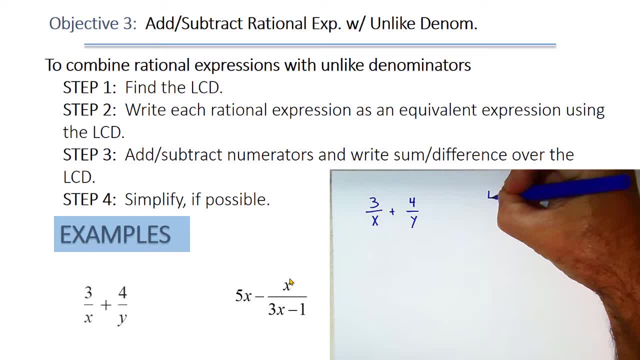 What is our common denominator there? Well, our common denominator is going to have to contain an x and a y. so that means our LCD is going to be the nice simple xy here. So we've already got the x in the fraction on the left. let's multiply top and bottom by y. 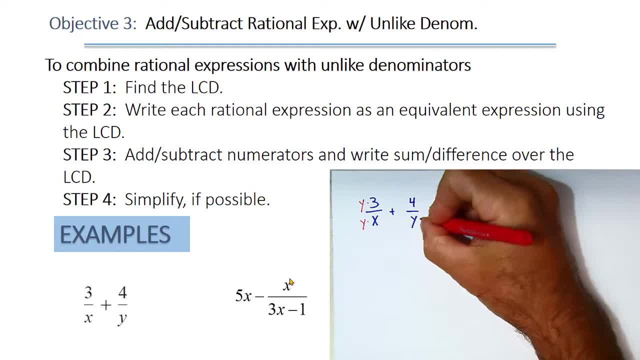 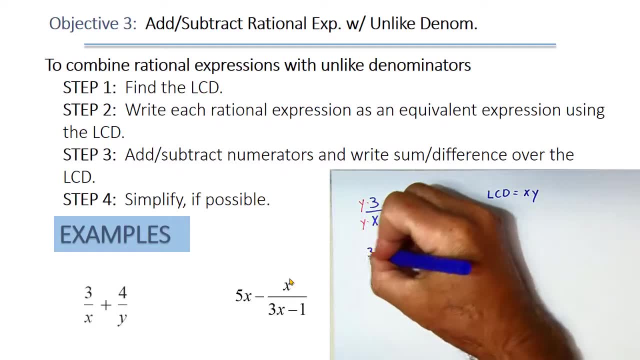 And on the right we already have the y. let's multiply in On top and bottom an x. Now that means that, although we wouldn't have to rewrite this, this problem is now 3y over xy plus 4x over xy. 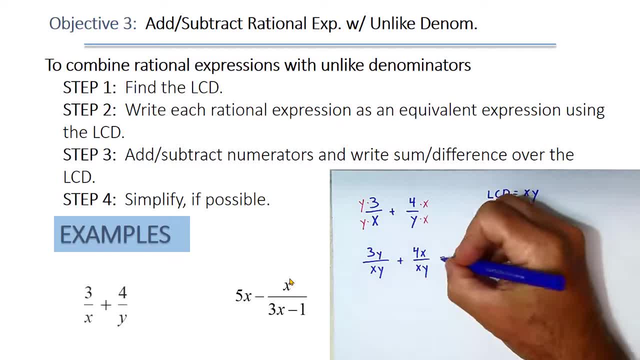 We have that common denominator so we can put the numerators together and that becomes 3y plus 4x. those are not like terms, so they can't go together, but they're both over xy. Now can we simplify that? 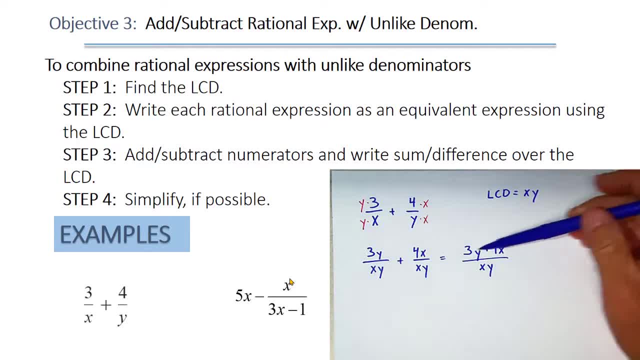 Does the top factor? Well, there's no GCF there, so, no, it doesn't look like anything factors at all, which means the only thing that we have here are terms. nothing cancels, and so that is our result. Now let's take a look at one more here. 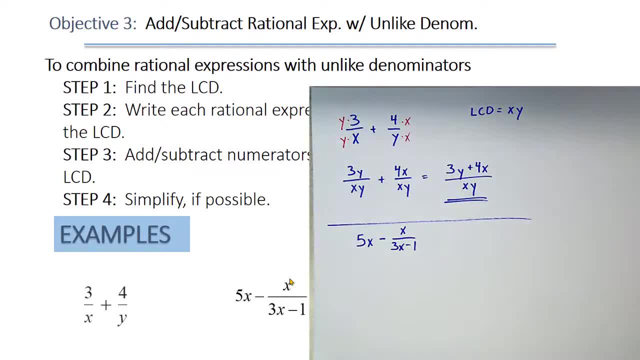 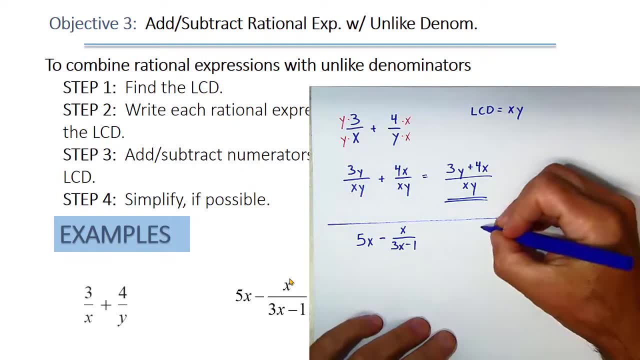 5x minus x over 3x minus 1.. Well, the term on our left, 5x- that doesn't even contain a fraction, so we could say that it's like 5x over 1, or we can simply say that our LCD here is 3x minus 1.. 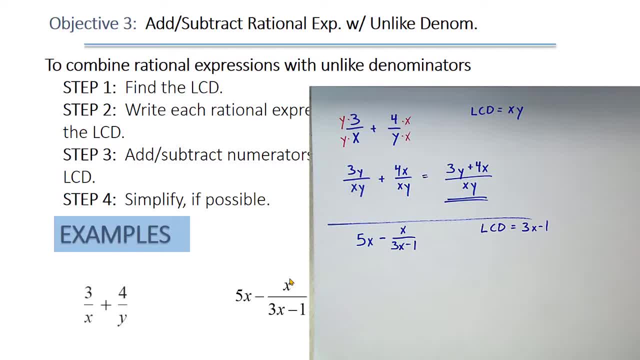 The only denominator here is the common denominator. That means we're going to rewrite this fraction on the left as 5x times 3x minus 1 over 3x minus 1.. Multiplying that 3x minus 1 into the top and bottom doesn't actually change the value of the fraction. 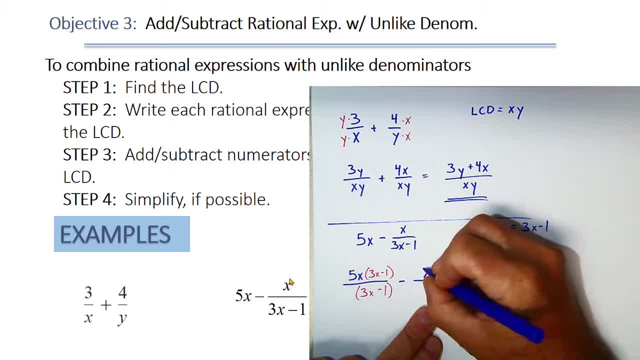 just the way it looks: Minus x over 3x minus 1.. We now have that common denominator, So we want to combine these numerators, but we can't do that until we distribute it in the 5x here. 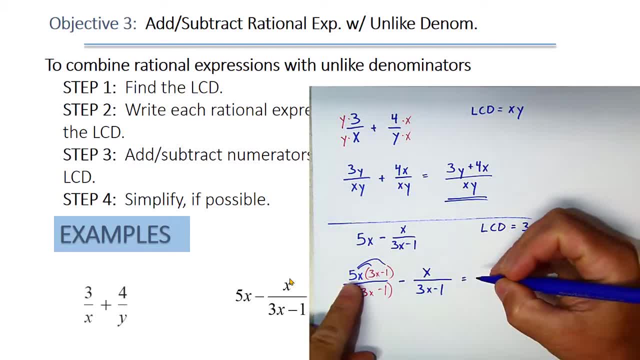 So if we distribute that in, we get 5x times 3x, that's 15x squared, And 5x times negative. 1 is minus 5x. And then finally the minus x from our second term. 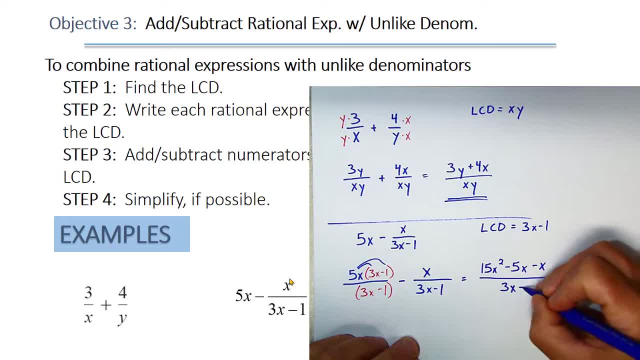 Those are now all over our common denominator of 3x minus 1.. So we can combine a couple of like terms in our equation. So we have our numerator here and that becomes 15x squared minus 5x minus x, that's minus 6x over 3x minus 1.. 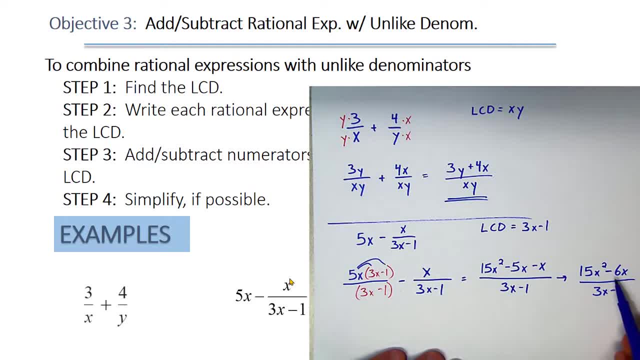 Now can we simplify that? Well, let's factor the top here, And the top does have a common factor of 3x in both of these terms. So it becomes 3x times 5x minus 2.. And that's all over: 3x minus 1.. 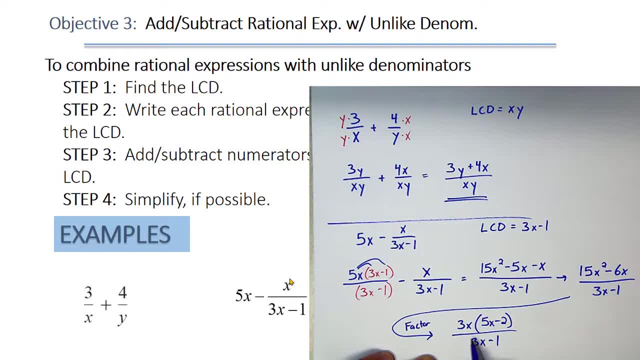 Now, do those 3x's cancel? Well, the top one would. That's multiplied on, but the bottom one does not. It's a term, And so that is where we would stop. And that raises the question: what if you would have quit back here. 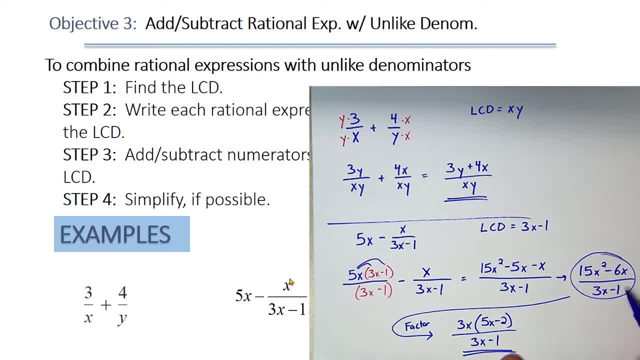 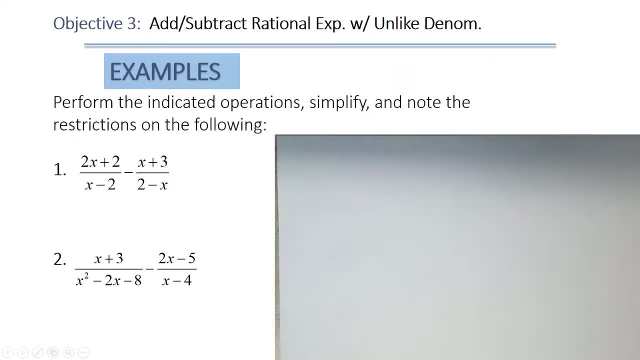 Well, that would be okay. So that turns out to be a correct solution, even though we don't really know it until after we've tried to factor and cancel. Let's take a look at two more quick examples Here to look at some sort of unusual cases, before I give you some for practice. 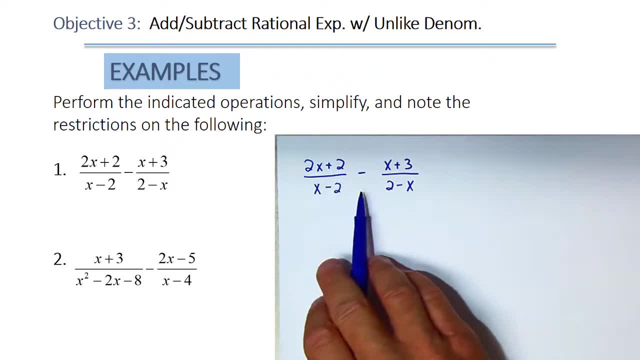 Our first one: 2x plus 2 over x minus 2 minus x plus 3 over 2 minus x. First question here is: are these two denominators the same or not? Well, if those were addition signs, they would be, because it wouldn't matter what order we add things. 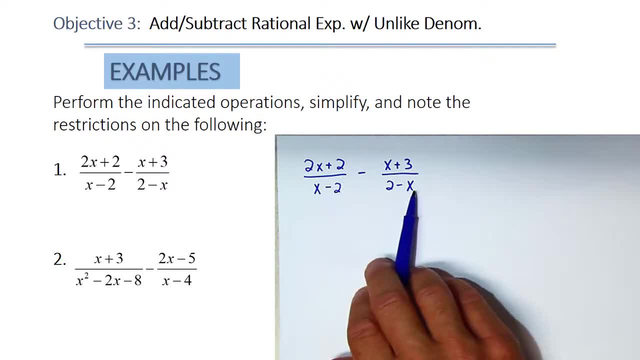 But these are subtraction signs. Is x minus 2 the same as 2 minus x? No, they're not. So these denominators are not the same, But we saw in our lesson yesterday that these are opposite binomials. We can make these two things the same. 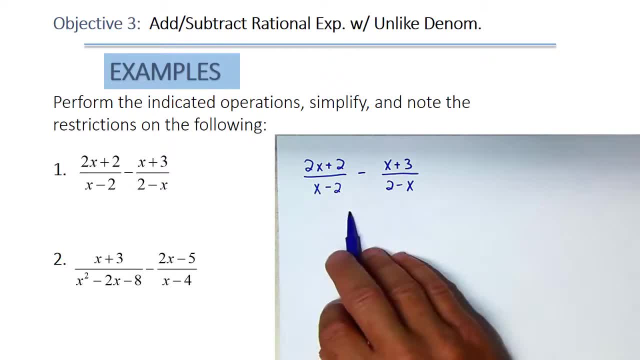 And we do that by factoring a negative sign out of one or the other. Now we could factor the negative sign out of the one on the left. That would make it match the one on the right, But let's factor out the negative sign for the one on the right. 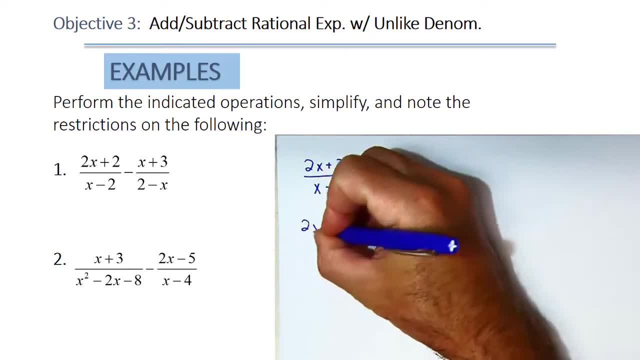 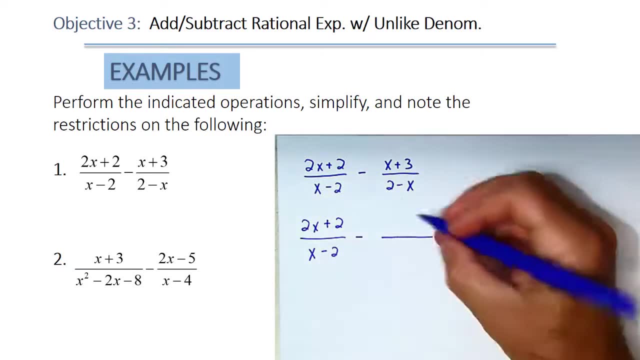 That's going to provide an advantage that you may or may not already see. So we're going to leave the fraction on the left as 2x plus 2 over x minus 2.. And the fraction on the right: I'm going to factor out a negative 1 out of that denominator. 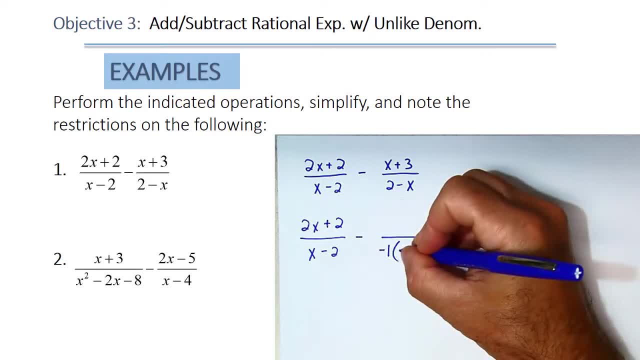 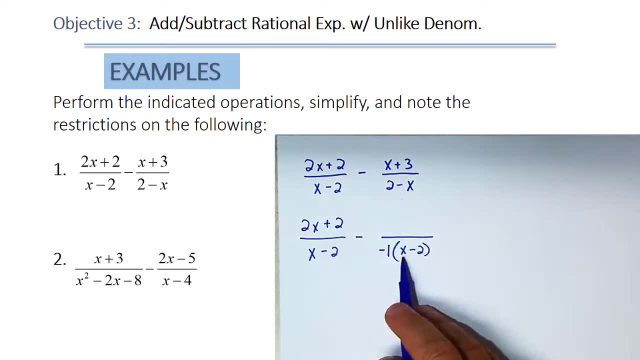 And if I factor out a negative 1, that becomes a negative 2 plus x, But I'm going to write that as x minus 2.. I want to make sure that you see the negative x becomes positive and the 2 becomes negative because we factored out a negative 1.. 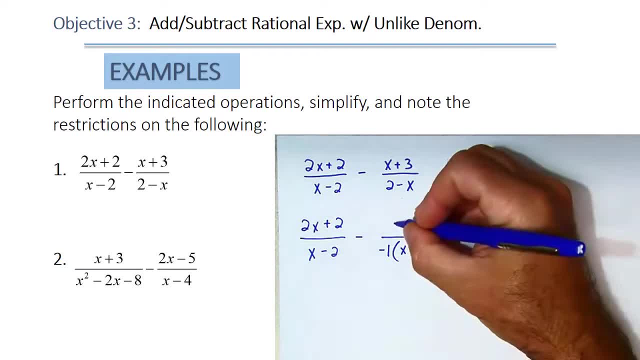 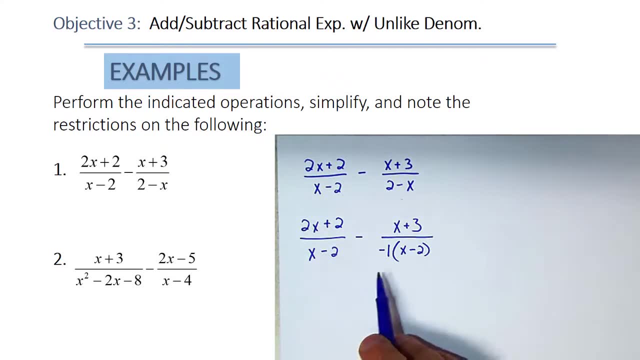 If I distributed that back in, we'd end up right back where we were, And of course the x plus 3 on the top does not change. So now we could say: okay, Our common denominator. Our common denominator has to contain an x minus 2 and it has to contain a negative 1.. 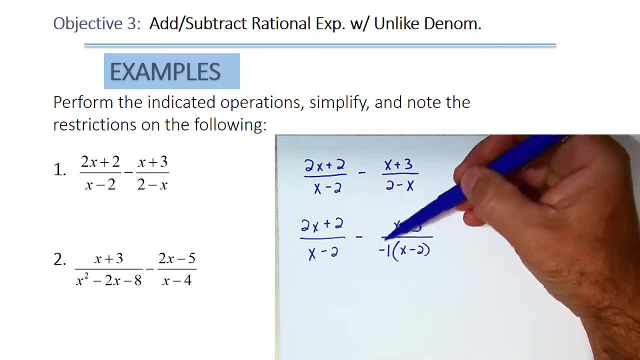 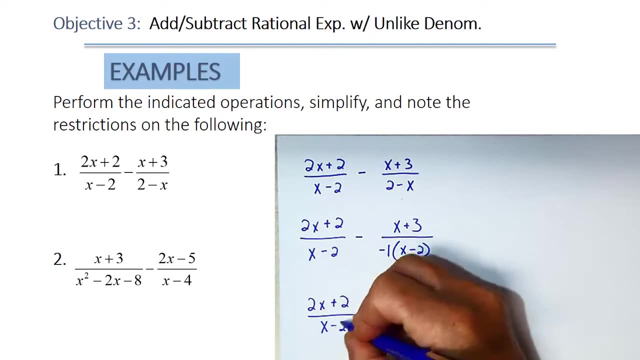 But keep in mind that if the top or bottom of a fraction is negative, it makes the whole thing negative. So we're really subtracting a negative fraction here. These two negative signs really combine to become a positive. So this becomes 2x plus 2 over x minus 2, plus these two team up. 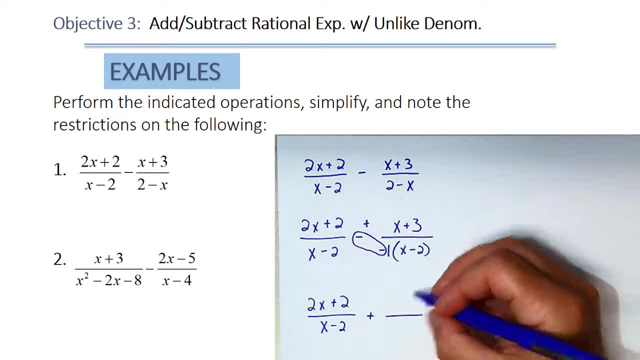 To become positive. And this is now x plus 3 over x minus 2.. Now, because of those opposite binomials, we factored out the negative sign. That really just changed our operation. But now we have the same denominator. 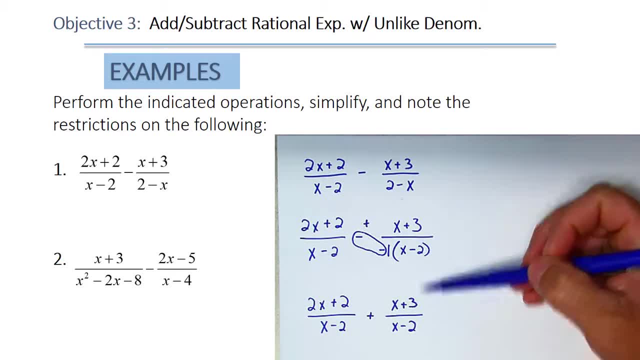 Go back and watch that explanation one more time if necessary to make that make sense. But we can run with this now. We can combine these two and say that we have 2x plus x, That's 3x And 2 plus 2.. 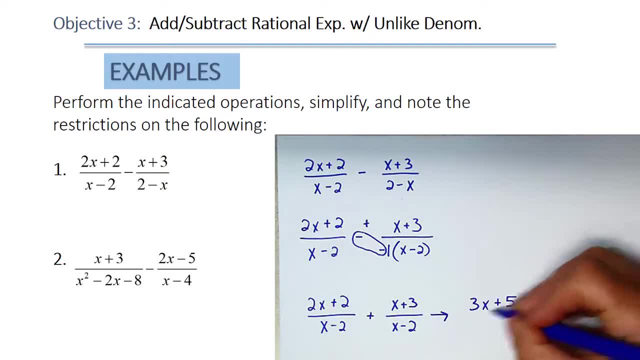 And 2 plus 3. That's 3x plus 5 over our common denominator of x minus 2.. Now we may or may not be done. Does the top factor? No, there's no GCF there. Nothing factors and therefore nothing cancels. 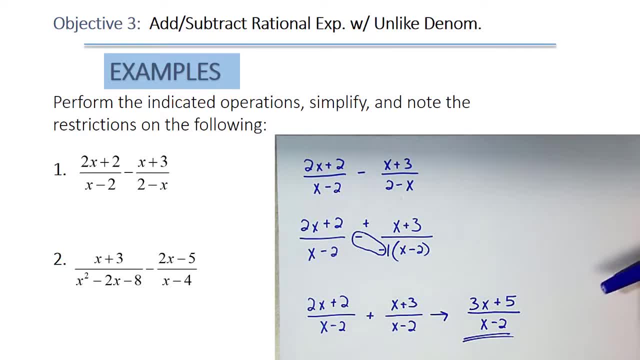 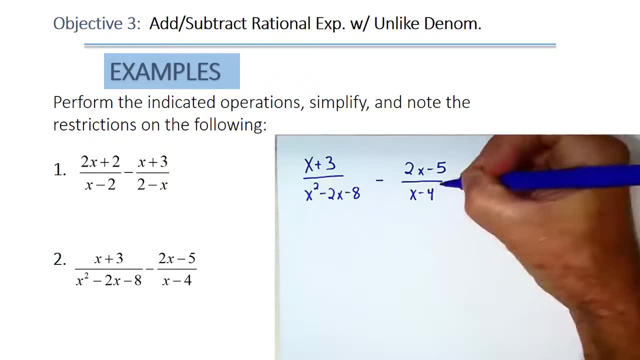 And we've performed that subtraction. Now I want to do one more with you as well before I give you some practice. Okay, So for starters, What's the common denominator here? We don't know until we factor everything right. 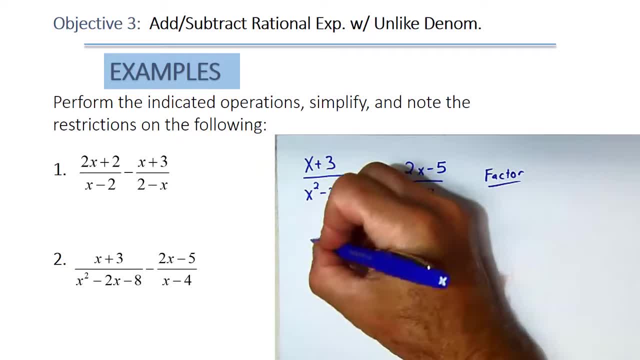 So let's get everything factored and then we can find our LCD. So our fraction on the left becomes x plus 3 over. That's a simple trinomial, and so that's going to be x minus 4 times x plus 2.. 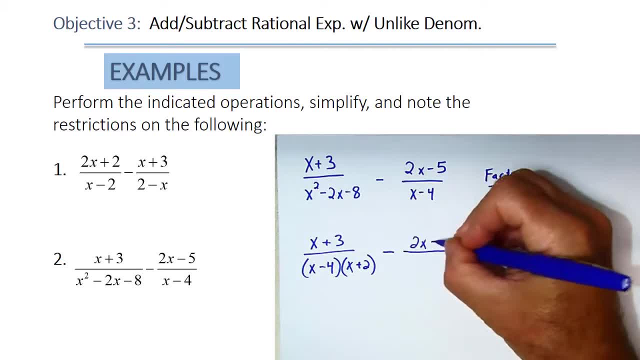 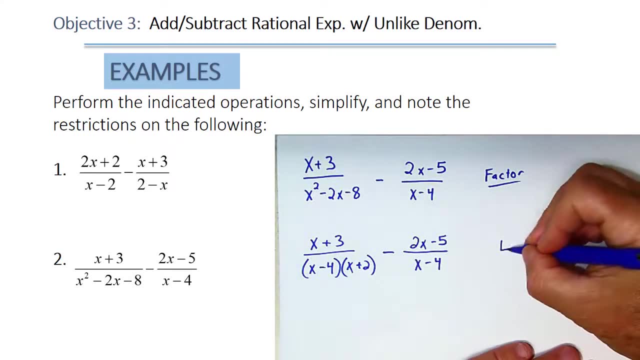 Minus the fraction on the right, There's really nothing to factor. That's 2x minus 5 over x minus 4.. Okay, It's pretty easy to see what our LCD is. So let's write that in: Our LCD has got to contain an x minus 4 and it also has to contain x plus 2.. 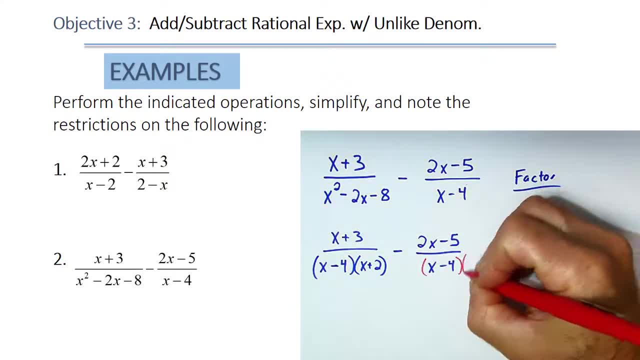 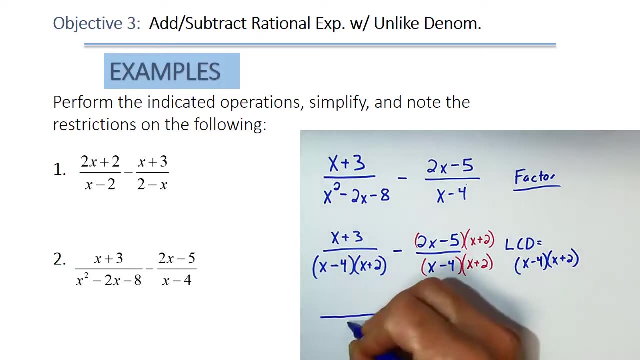 So that means this fraction: on the right we need to multiply in the factor of x plus 2. on the top and the bottom We'll use parentheses, so we're sure to FOIL in our next step. So now we can express these all over our common denominator of x minus 4.. 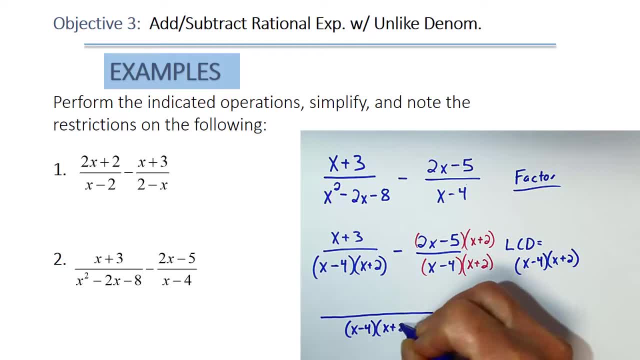 So we have x minus 4 times x plus 2.. Okay, We have x plus 3 from the left fraction, and now we're going to subtract off the product of our FOILing. on the right. We have 2x times x. 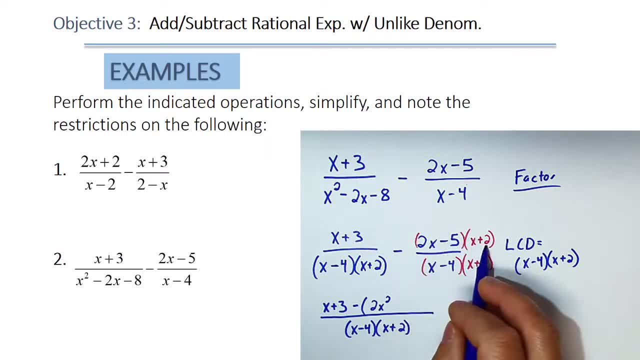 That's 2x squared and 2x times 2. That's plus 4x on the outside but minus 5x on the inside. So that's minus x and negative 5 times positive. 2 is negative 10.. 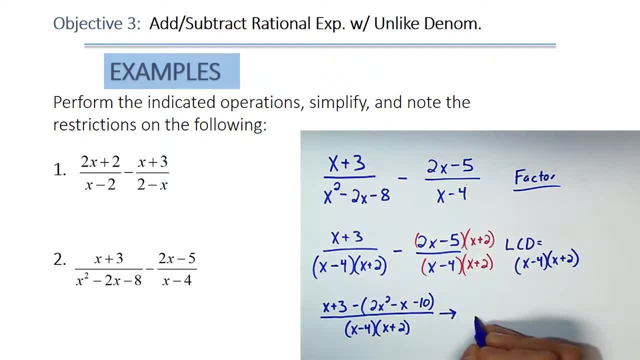 Now we can simplify that numerator by combining like terms. We'll do some of this in one step. here We've got a negative 2x squared. When we distribute that negative sign, that'll give us a positive x. but we had another x out front, so that's plus 2x. 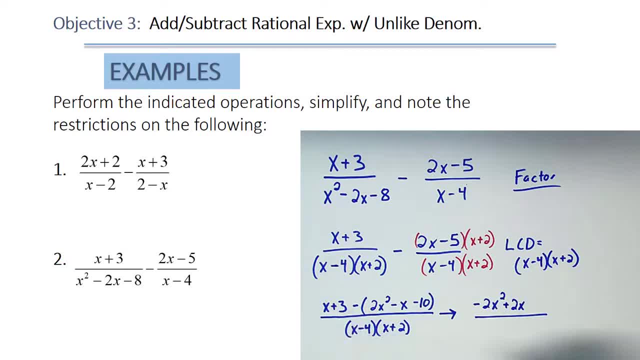 We also have a negative times, negative 10.. That's positive 10 plus the 3 in front, That's positive 13.. And that's now over our common denominator of x minus 4.. That's our common denominator of x minus 4 times x plus 2.. 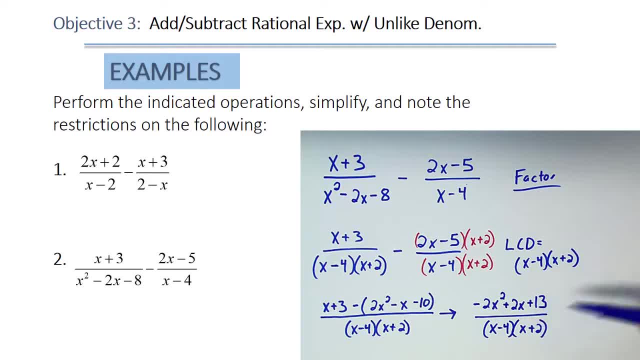 Now let's see if the top factors, if the top factors, we might get some cancellation. Let's do our factoring test by grouping. Take negative 2 times 13. That's negative 26.. Are there two factors of negative 26 that add up to 2?? 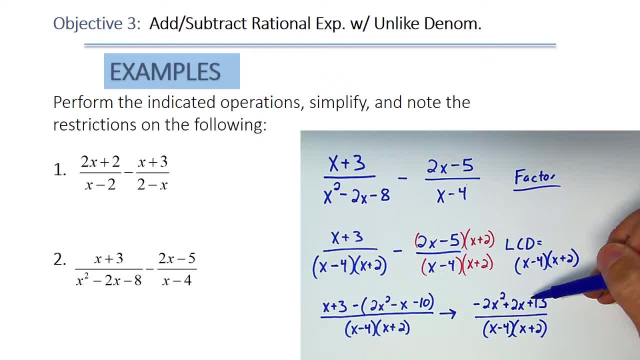 If so, we can split up that middle term and factor by grouping, But no Negative 2 times 13, which is negative 26. That can't be broken into two factors that add to 2. The top must be prime and therefore it won't factor, and that means that this is our final result. 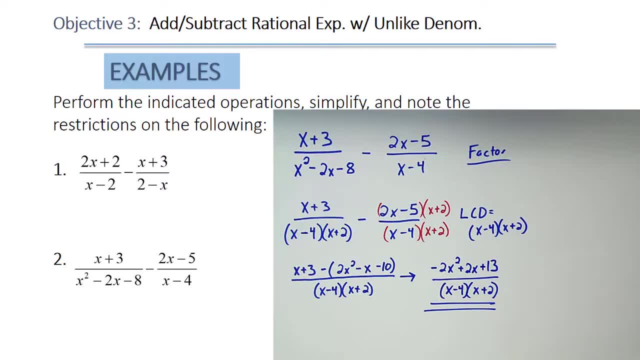 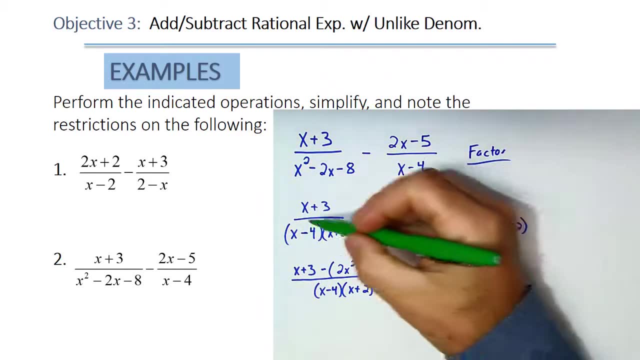 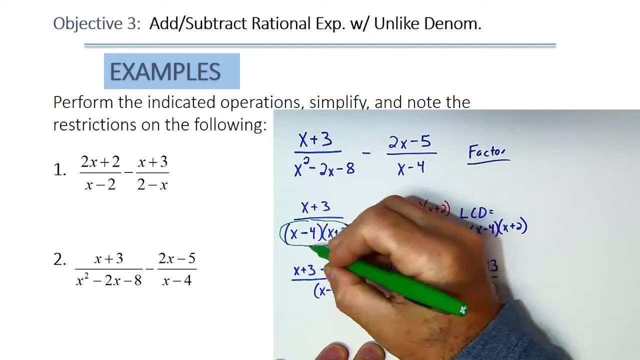 Now we're still not quite done, because this problem also asked us to find our restrictions on the variable. So if we go back to our original problem after we did our factoring, at that point we can stop and recognize the restrictions. So in this denominator, x minus 4 times x plus 2,. 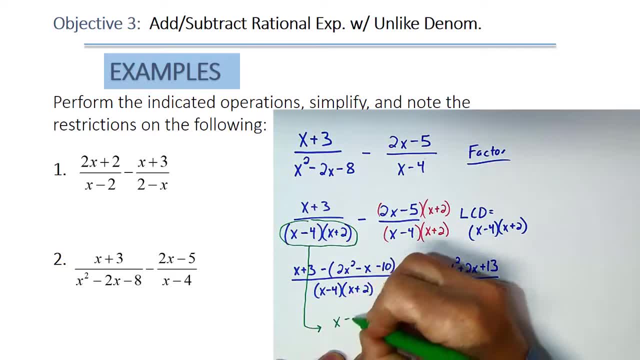 we can recognize that neither of those factors can be 0. So x minus 4 cannot equal 0. And that means x is not allowed to be 4.. And the other factor there, x plus 2, that can't be 0.. 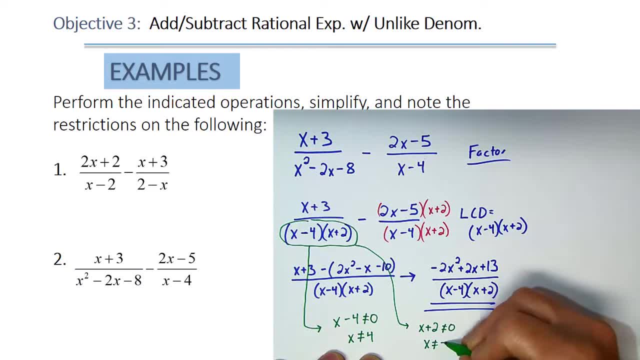 And therefore, if we subtract 2, we can see that x cannot be negative 2.. And so there's our two restrictions. Now, on the right, we also had a denominator of x minus 4.. So that would be another restriction, except for we already covered that case. 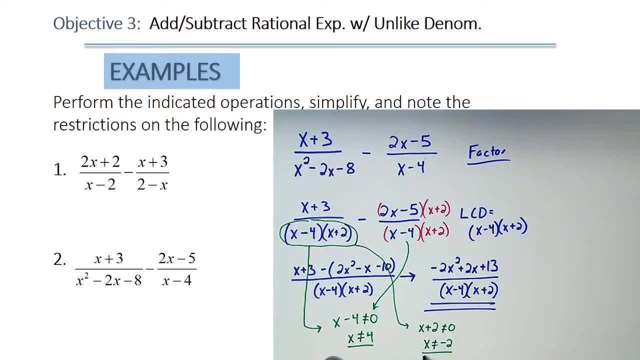 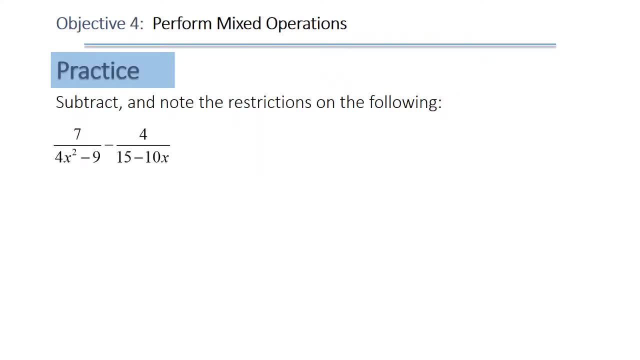 And so we don't need to cover it again. Our restrictions are: x cannot be negative, 2 and x cannot be 4.. Okay, I'd like you to try one for practice here. There's a problem on your screen. Figure out what the common denominator is there and perform that subtraction. 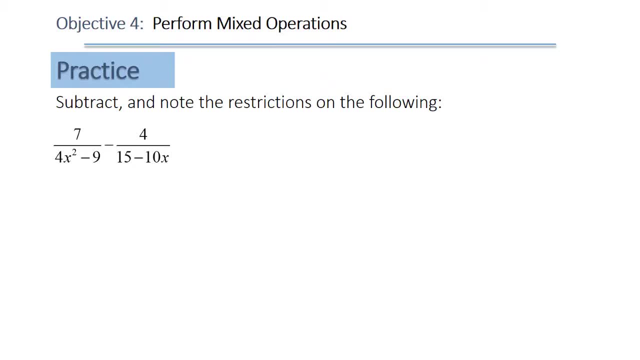 This time, just as a little refresher, note what the restrictions are on your fractions as well. Go ahead and do that and unpause when you're ready to see that solution. Okay, so right off the bat, here we know we're going to have to factor these denominators. 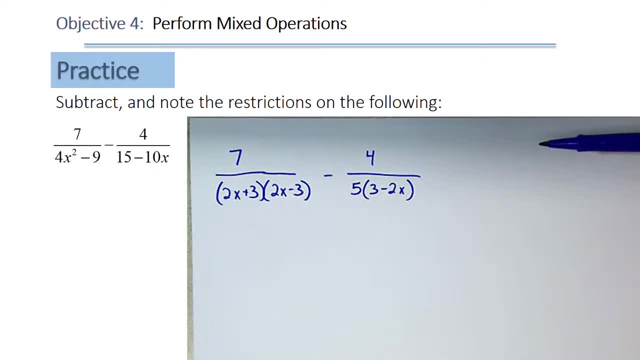 I'd like to factor those as soon as I write the problem down and save some writing. So the left denominator factors the difference of squares and the right denominator has a GCF of 5 that we can pull out. So what is our common denominator here? 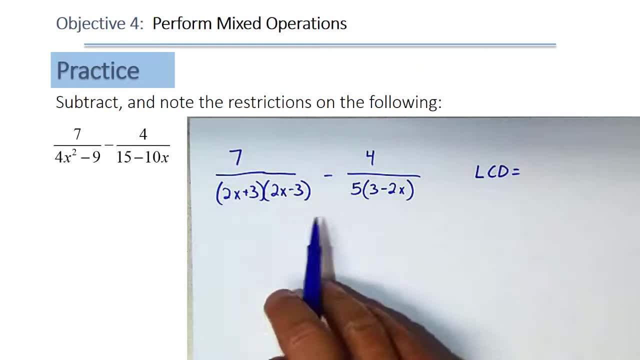 What is the LCD? Well, look at this. We know we need to have a 5, and we know we need to have a 2x plus 3.. But do we need a 2x minus 3 and a 3 minus 2?? 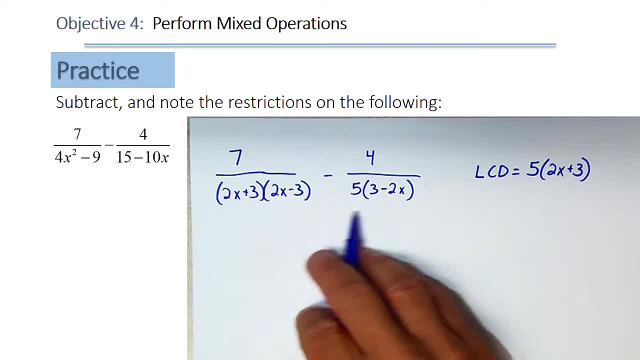 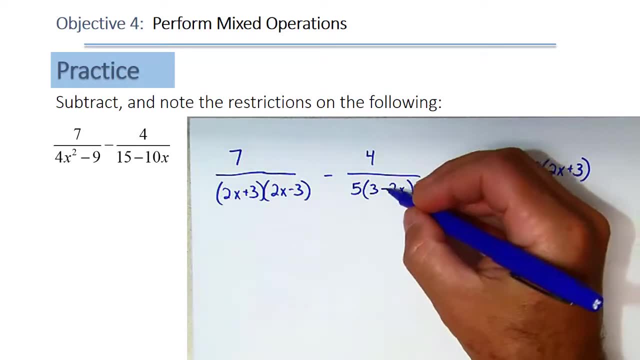 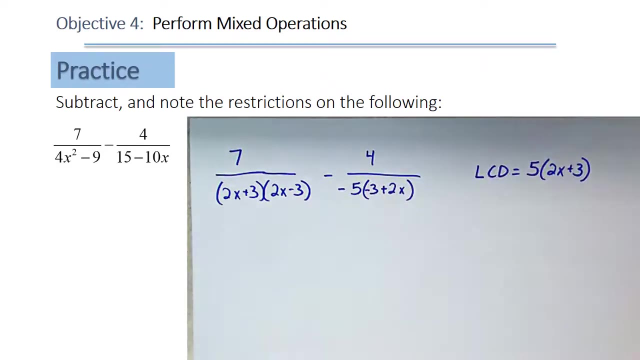 Not really, because we could make this 3 minus 2x match the 2x minus 3 if we factored out a negative 5 instead. So if we factor out a negative sign with that, that becomes a negative 3 and a plus 2x. 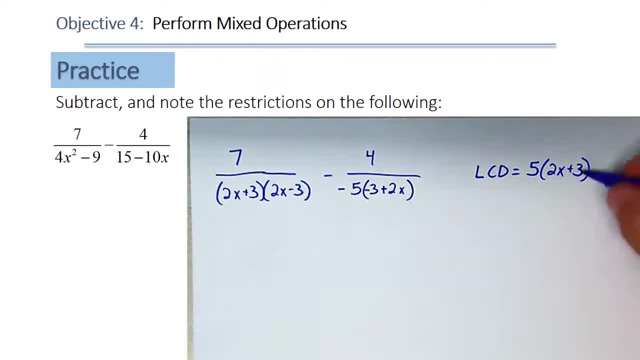 Now we have 2x minus 3 on both of these, So our other factor is 2x minus 3.. And you might say, well, now we need a negative 5 in our LCD. Nope, that can stay 5, because what are we going to do with that negative sign? 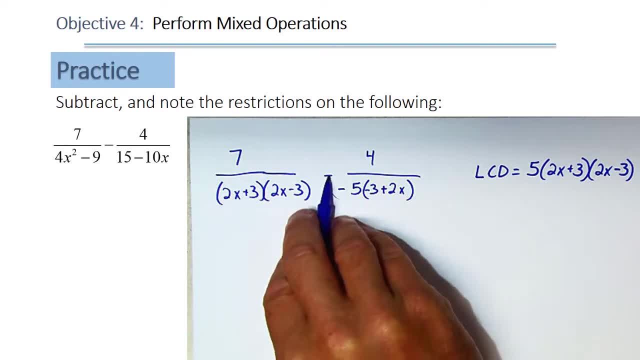 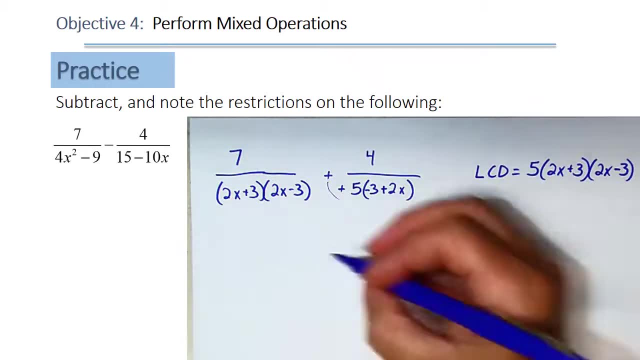 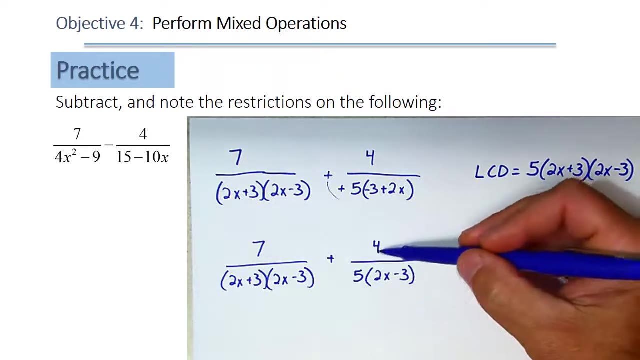 We'll make it team up with the one that's already there. If this would have been positive, then this would simply become a subtraction problem, But those two cancel off And the new problem that we're looking at is 7 over 2x plus 3, 2x minus 3, plus 4 over 5 times 2x minus 3.. 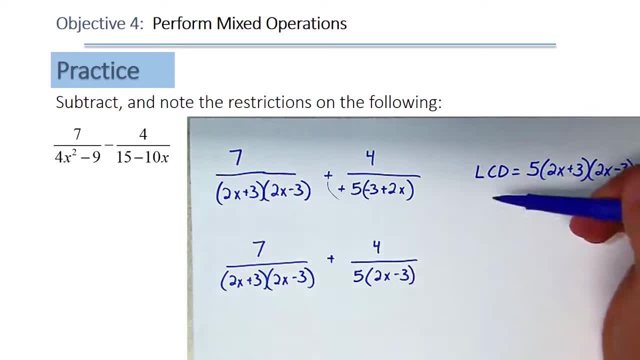 We reversed the signs on that binomial and that changed the operation to addition. So let's figure out what our missing factors are. For our fraction on the left, we just need to multiply in a factor of 5 there. I'm going to do it on the edge right there. 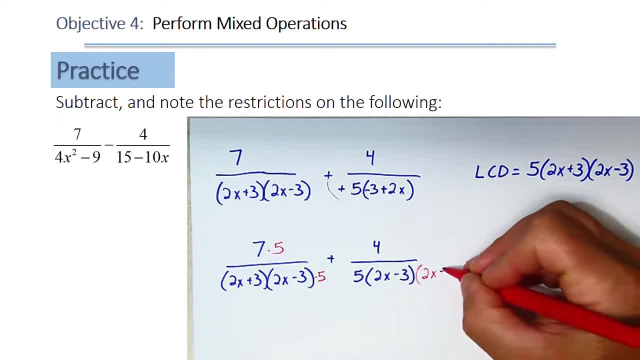 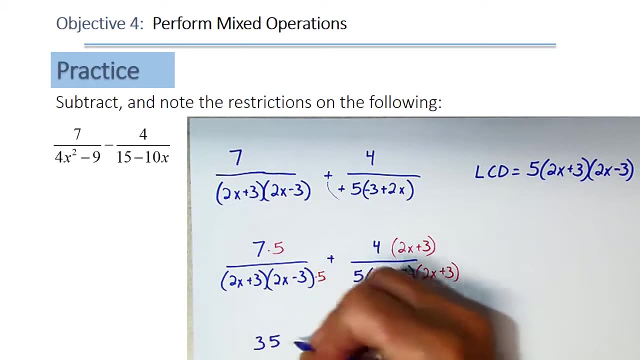 And for the fraction on the right, we have to multiply in 2x plus 3.. Okay, and that allows us to have a common denominator. so now we can combine our numerators. This becomes 35 plus 4 times 3.. 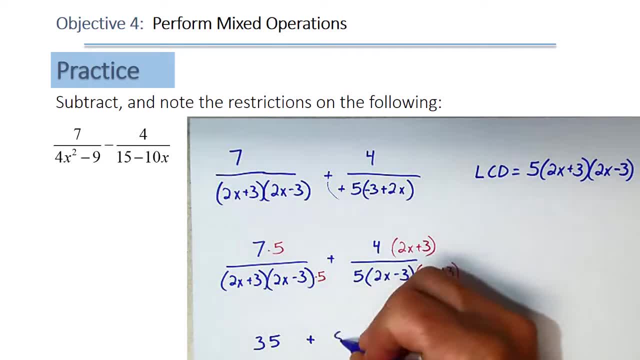 4 times 2x, that's 8x, And 4 times 3,, that's plus 12.. And those are now combined and all over our common denominator. Now we can go a little bit further with that, because we have a couple like terms here. 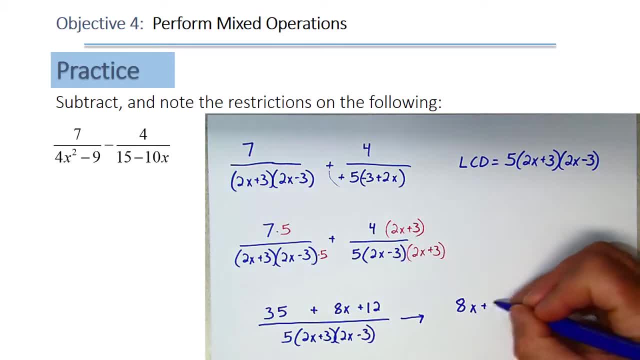 We can call that 8x plus 47, all over our common denominator of 5 times 2x plus 3 times 2x minus 3.. And since that numerator doesn't factor at all, nothing will cancel and we're done. 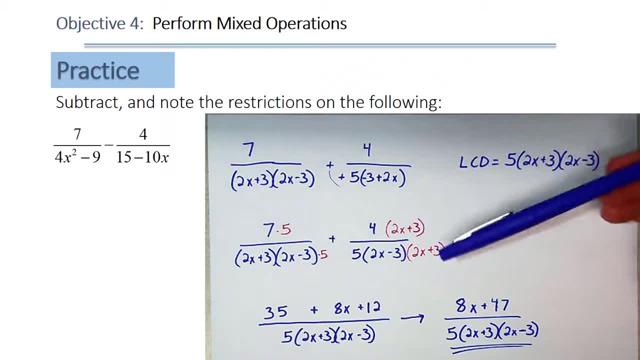 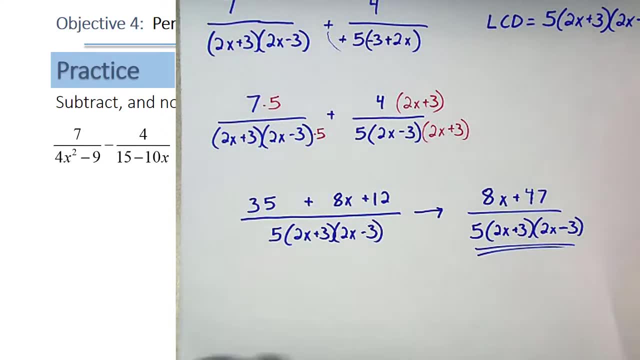 If you got that great job. There's a lot going on in that problem. If not, make sure you rewind to learn from any mistakes you may have made. Now let's note our restrictions here. We already noted that the common denominator contained a 5, a 2x plus 3, and a 2x minus 3.. 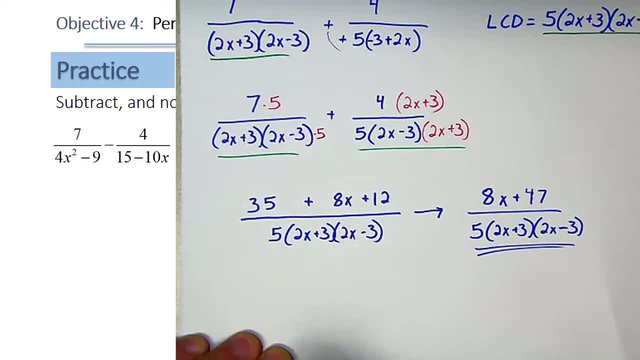 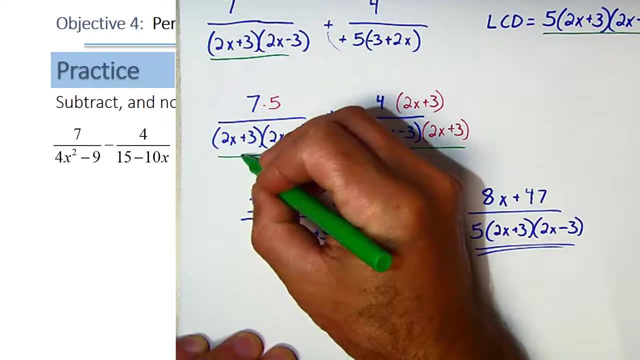 We can see that in several places. So if we look at each of the factors in our denominator, we can see what our restrictions are. The first one: 2x plus 3, that was one factor. So we can note that 2x plus 3, that's not allowed to be equal to 0. 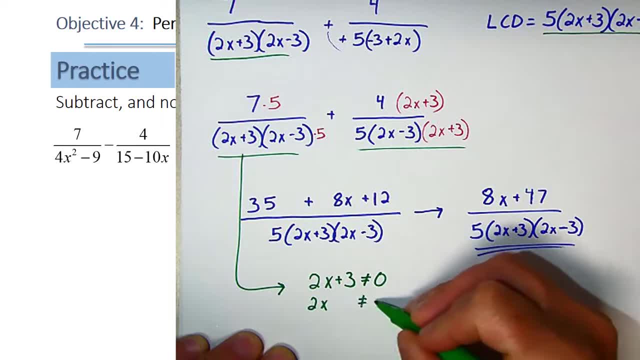 Subtract 3 and we can see that 2x is not allowed to be equal to negative 3.. And then divide by 2 and it reveals our first restriction: x cannot be negative, 3 halves. So that's one value of x that we simply can't put into this expression. 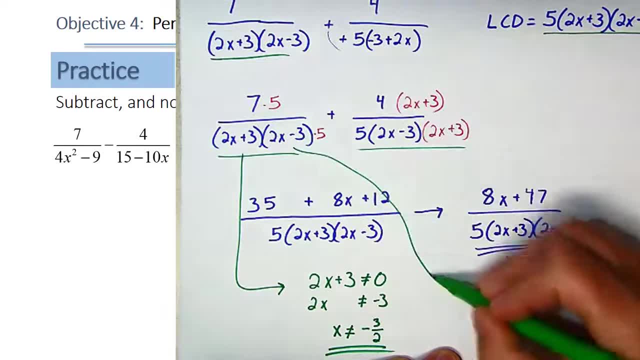 And then the other one is 2x minus 3, that can't be equal to 0. And the math there is going to be very similar: If 2x minus 3 cannot be equal to 0, we'll add 3 to both sides to see that 2x cannot be equal to 3.. 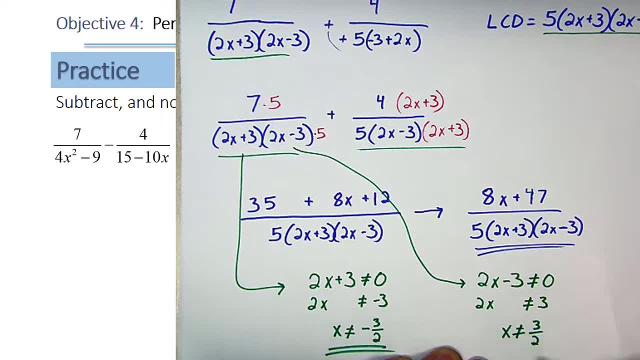 Divide by 2, x cannot be equal to 3 halves. And there's our other restriction. Now you could say, well, there's a factor of 5 here. That's true, but kind of like when we were using zero product property, that's never going to equal 0. 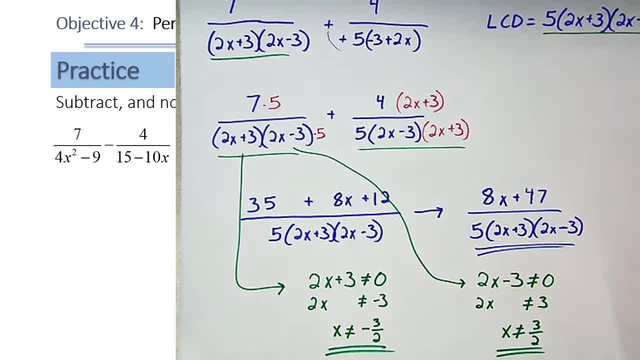 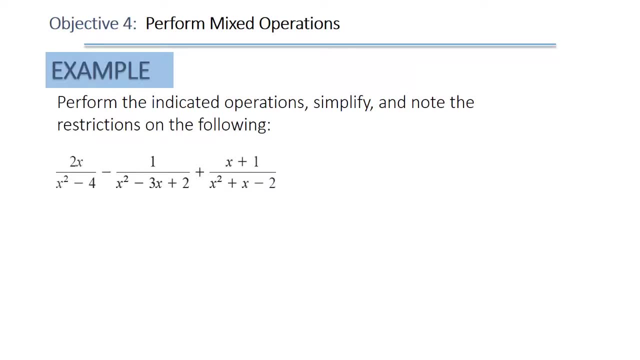 5 is equal to 5, and so there's nothing variable about that. It's not going to yield a restriction. Negative 3 halves and positive 3 halves are the two restrictions. Okay, let's take a look at one more real, tricky one. 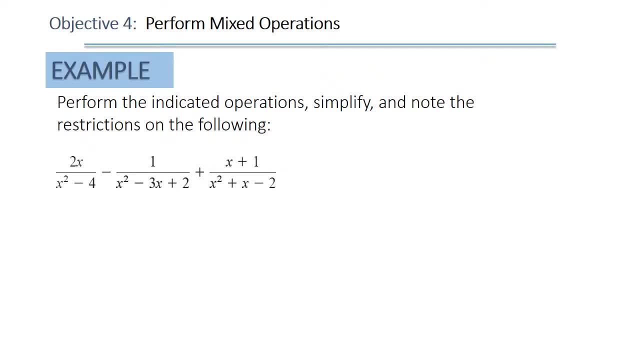 And if you can do this one, you're in real good shape. We'll work through this one together and then I'll give you one last tricky one to wrap up this lesson, Okay, well, as we did before, as soon as I write the problem down, 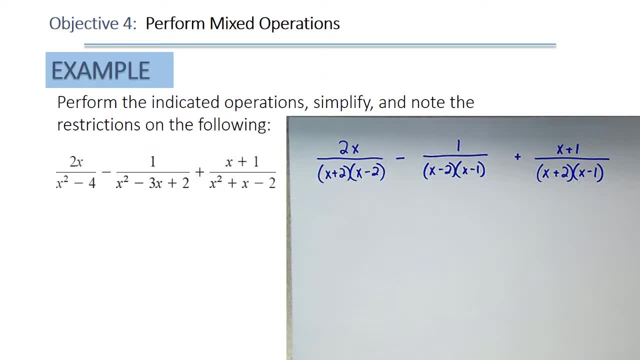 I like to do the factoring in the denominator, since we know that's our first step anyway. And so all three of those denominators factor. Now, what would your common denominator be? We're going to have to have an x plus 2, an x minus 2, and an x minus 1.. 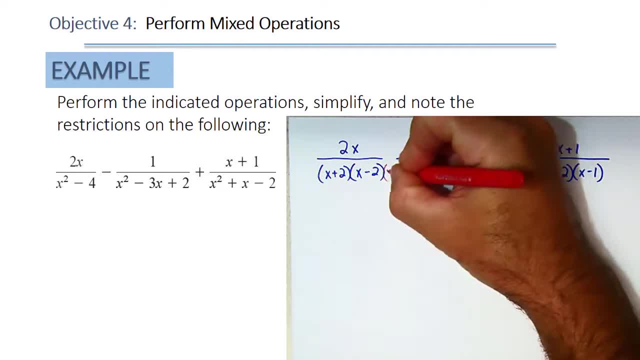 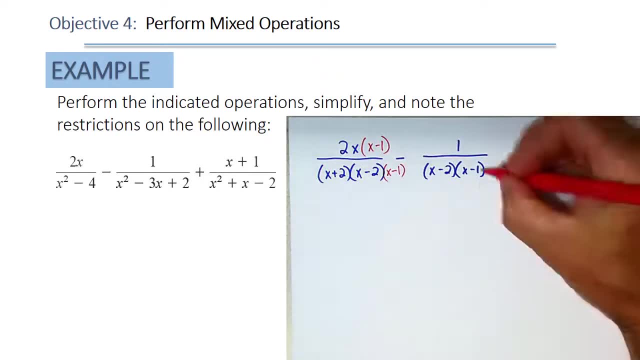 So we can fill in the missing factors. The fraction on the left is missing- the x minus 1 factor, Let's put that in. The fraction in the middle is missing- the x plus 2 factor. Let's put that in. And the fraction on the right is missing- the x minus 2 factor. so let's put that in. 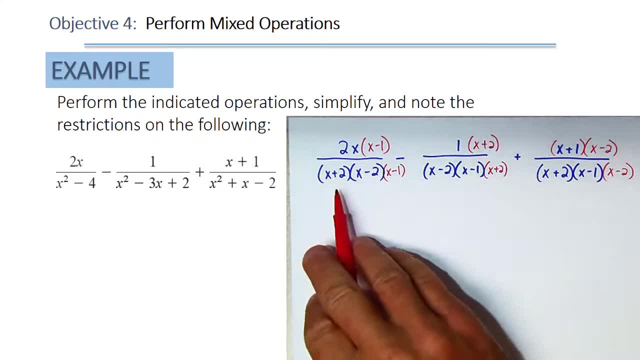 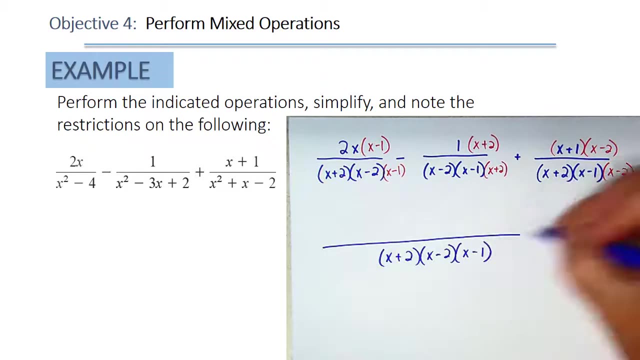 Now, when we do that, you can see that we have all three denominators the same: x plus 2x minus 2x minus 1.. And since we've now done that, we can go ahead and rewrite all those over, our new common denominator. 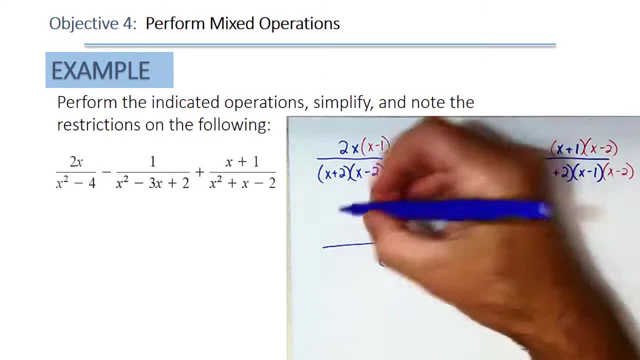 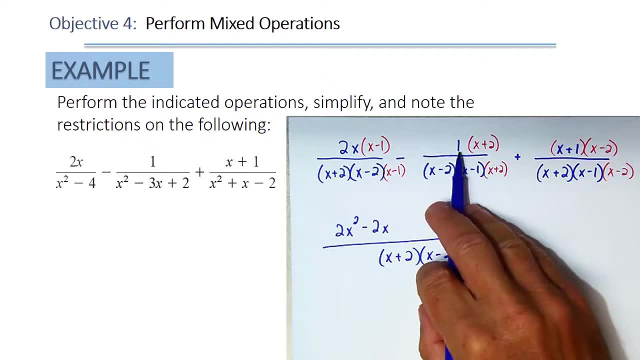 And once we've done that, in our top left we can distribute in the 2x. We get 2x squared minus 2x. Now in our middle numerator, we can distribute in the 2x. Now in our middle numerator, we can distribute in the 2x. 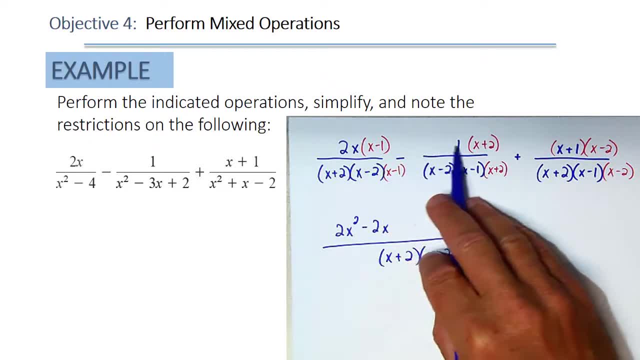 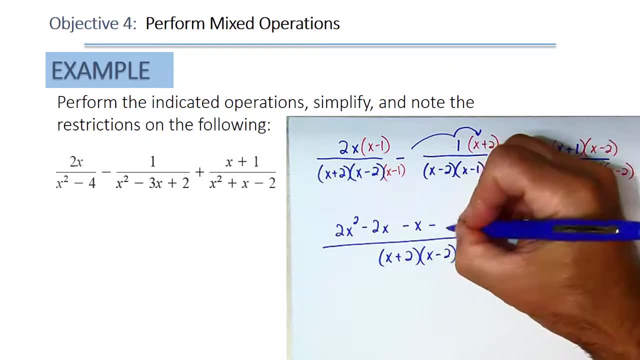 Now in our middle numerator we can distribute in the 2x. Remember that's subtraction. so we're going to distribute in a negative 1.. Negative 1 times x is minus x and negative 1 times 2 is minus 2.. 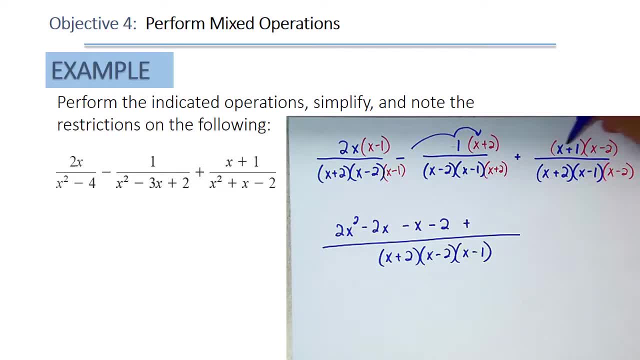 And on the right, we're going to add on the product of this multiplication or this FOILing. So that's going to be x squared minus 2x but plus 1x. So that's going to be minus x and plus 1 times negative. 2 is minus 2.. 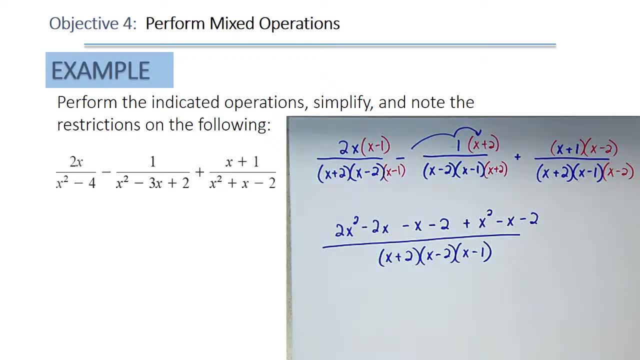 So let's combine our like-and-different factors, So let's combine our like terms there. But just to make sure that you're with me, we distributed in the left numerator, we distributed in the center numerator and we FOILed the right numerator to get all those terms. 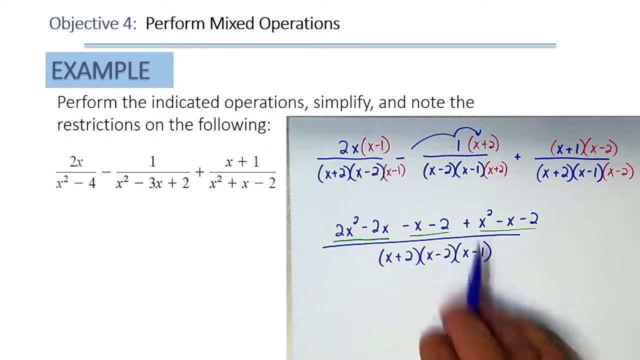 So if we combine any like terms, we have 2x squared plus x squared, That's going to be 3x squared minus 2x, minus x, minus x, That's minus 4x. And then we have negative 2 minus 2, which gives us negative 4, all over our denominator. 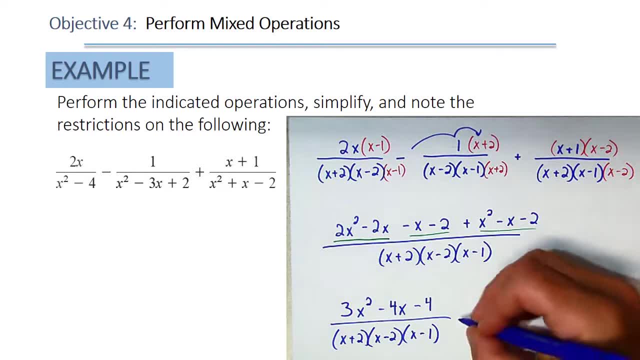 Now we may or may not be done. Let's see if this numerator factors at all. You could factor that by grouping 3 times negative, 4 is negative 12, which you could split into two factors. I'm going to trust that you could do that. 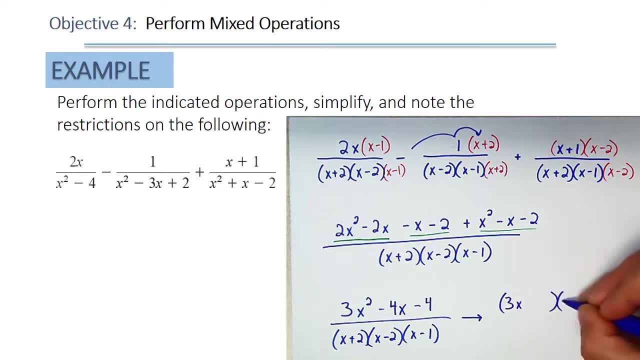 You could also factor this one by inspection. We can say: well, we know what has to be 3x and x in order to get 3x squared, And the logical choices to try here are 2 and 2 to get our last term of 4.. 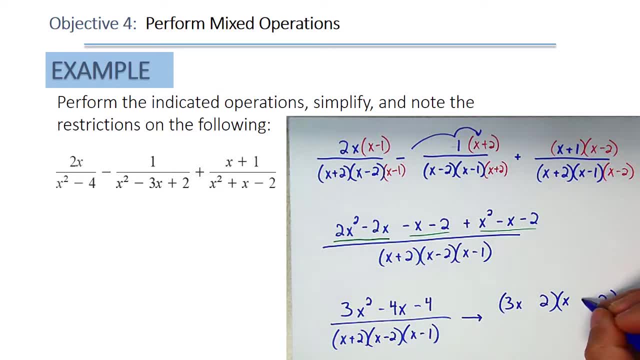 One will need to be positive and one will need to be negative. So if we make that 3x plus 2 times x minus 2, that is our factorization. Now in the denominator we still have the same factors: x plus 2,, x minus 2, and x minus 1.. 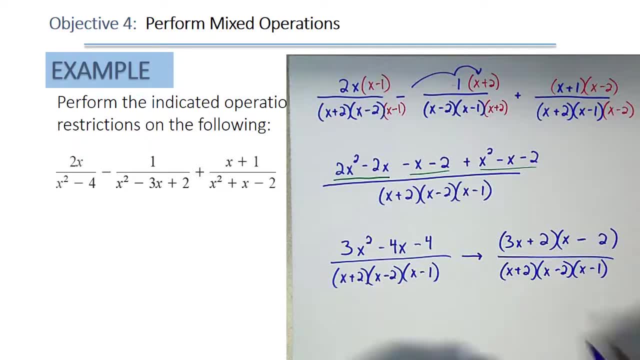 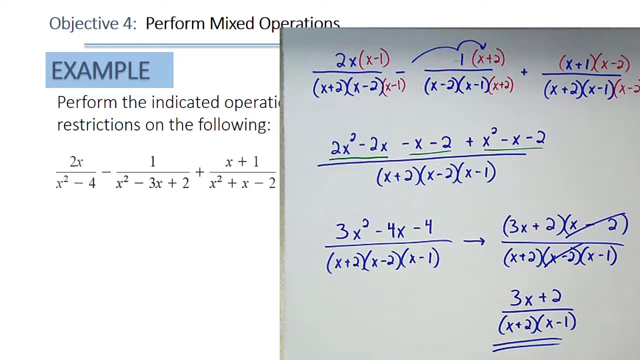 Now you'll probably note that we get some canceling there. So the x minus 2s cancel completely, And there's our final result: 3x plus 2 over x plus 2 times x minus 1.. And one more time: what were our restrictions here? 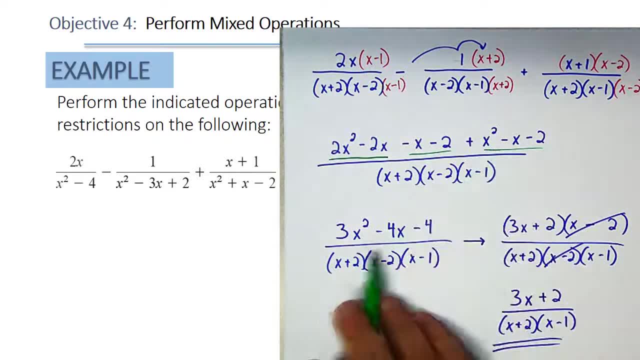 Well, we got a common denominator so we can look at any point along the way. But look at what your factors were in that denominator. We know that x plus 2 would not be allowed to be 0, and so x can't be negative 2.. 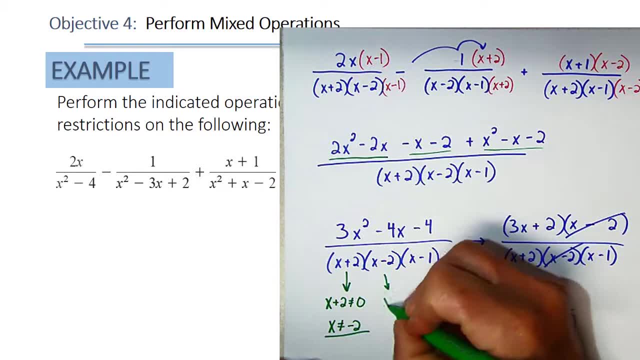 x minus 2 can't be negative 2.. x minus 2 can't be 0, and therefore x cannot be equal to 2.. And x minus 1 is our third factor in the denominator. That can't be equal to 0.. 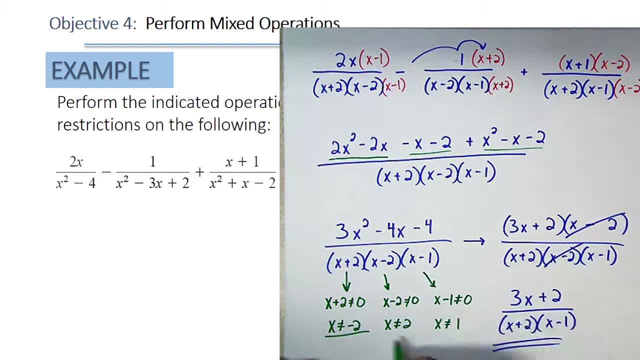 And if we add 1 to both sides, x cannot be equal to 1.. So this time we have three restrictions: x can't be negative 2,, 2, or 1 in this entire algebraic expression. Okay, and I want to give you one last one to practice here, one last tricky problem. 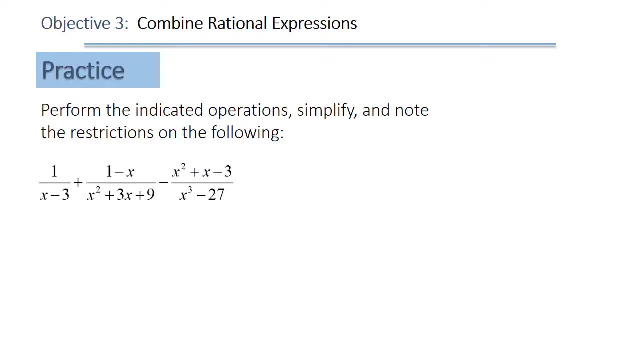 And if you can do this one, why You got it? So go ahead and work the one on your screen, Find the restrictions when you're done, Unpause when you're ready to see that solution. Okay, well again, let's factor everything right when we write the problem down. 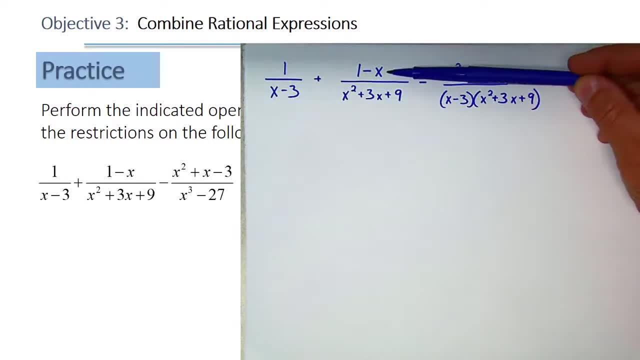 The fraction on the left. there's nothing there that factors In the middle. the top clearly doesn't factor. The bottom kind of feels like that denominator should factor. It's a trinomial, but it doesn't. As it turns out, that's prime. 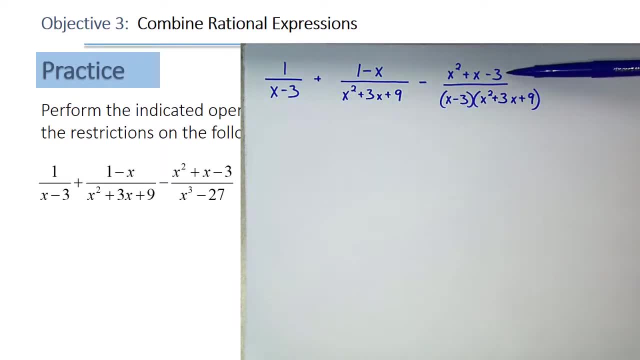 The fraction on the right. The top feels like it should factor, but it doesn't. But the bottom right is the only thing that factors here. x squared minus 27 should recognize that as a difference of cubes, And so that becomes x minus 3 times x squared plus 3x plus 9.. 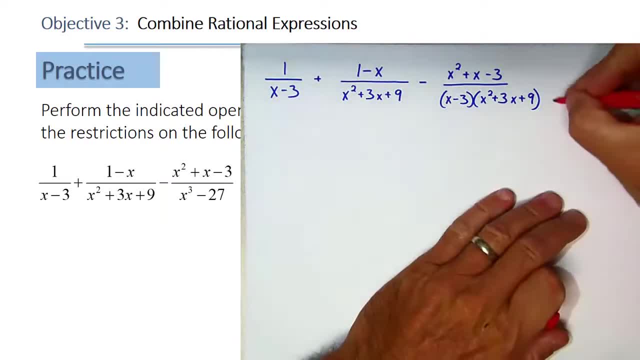 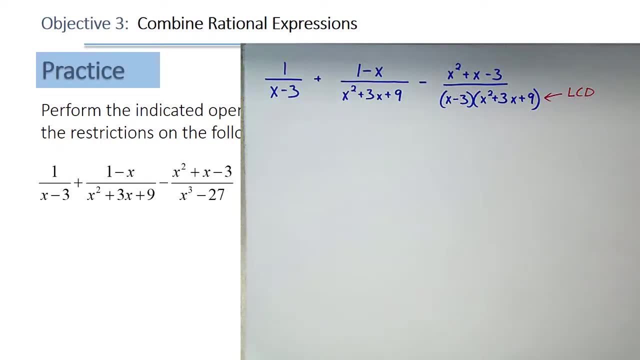 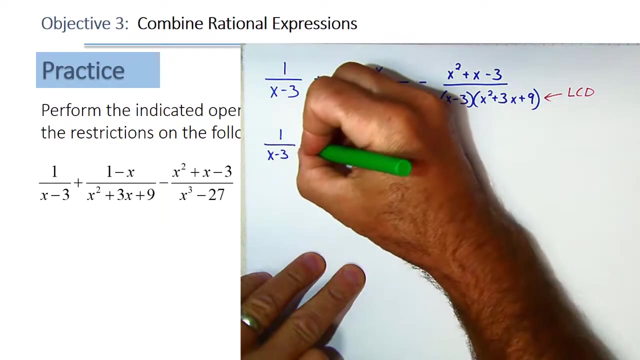 So what is our denominator? Well, as it turns out, that very last denominator, that is our common denominator, And so let's fill in the missing factors in our other two fractions, So the fraction on the left. we already have the x minus 3 in there. 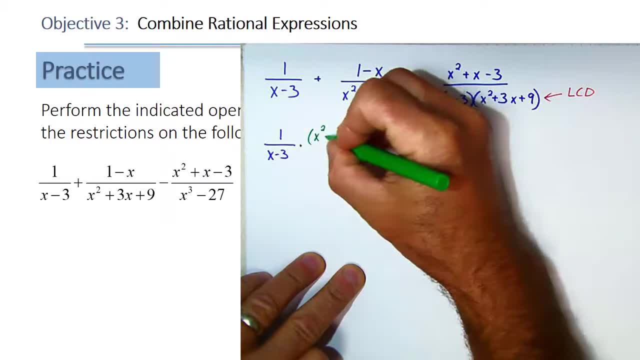 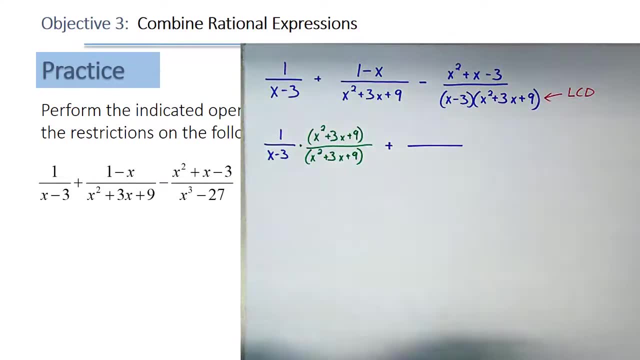 but we're going to multiply in both top and bottom: x squared plus 3x plus 9.. And to that we're going to add, on our second fraction, which we already have, the x squared plus 3x plus 9 in the denominator. 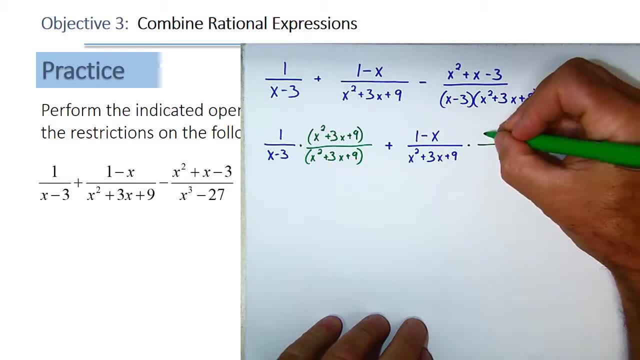 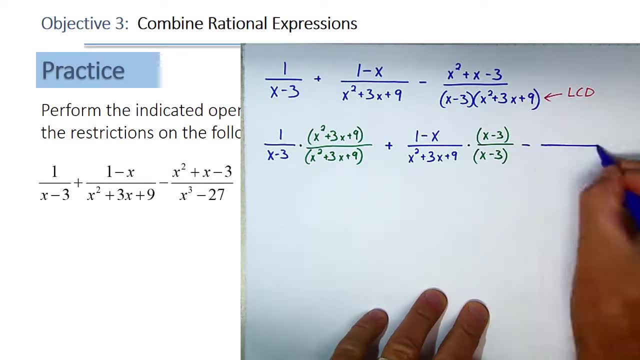 So this time we're going to multiply top and bottom by the missing factor of x minus 3.. And in our third fraction, there, well, we've got our common denominator, so there's no work to do So now that we've got the same denominator in all three of these. 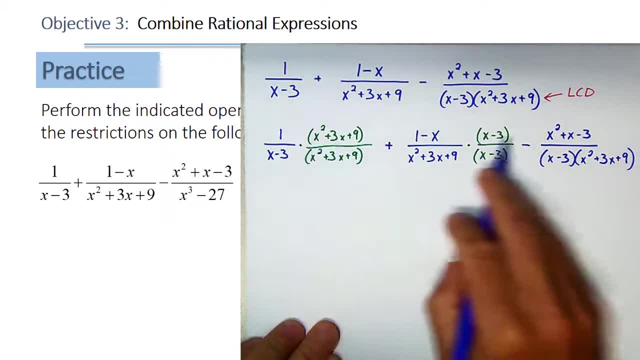 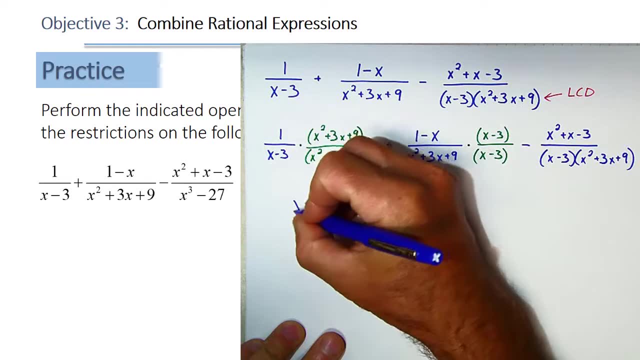 we can get to the work of combining these kind of messy numerators here. So let's start with this numerator on the left: 1 times x squared plus 3x plus 9.. That's simply going to be x squared plus 3x plus 9.. 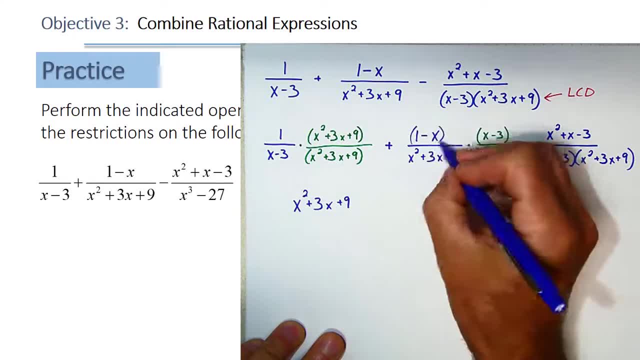 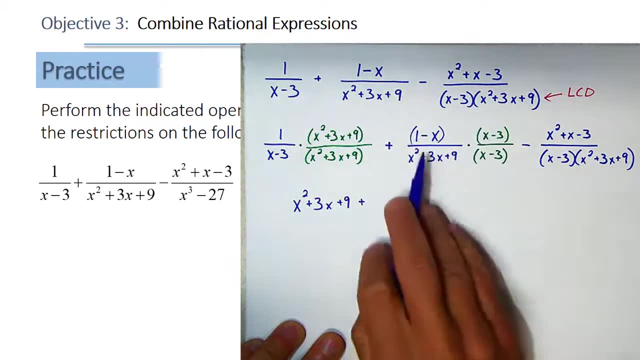 To that we're going to add the product of these two numerators: 1 minus x times the new x minus 3.. And if we FOIL that, that means that we're going to be adding in: 1 times x is x. 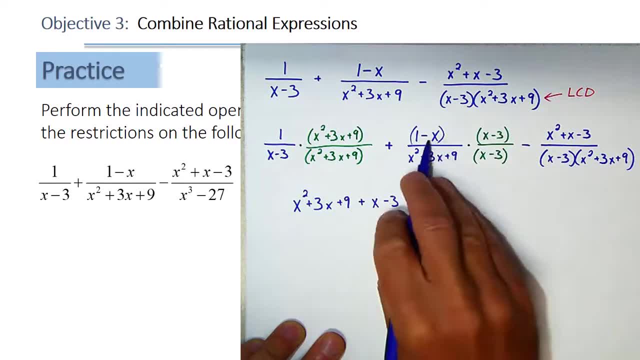 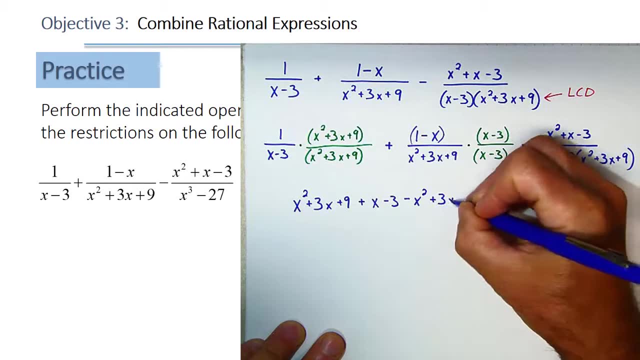 1 times negative 3 is minus 3.. Negative x times x is minus x squared, And negative x times negative 3 is plus 3x. And now we are going to have to distribute in the negative sign on our last numerator. 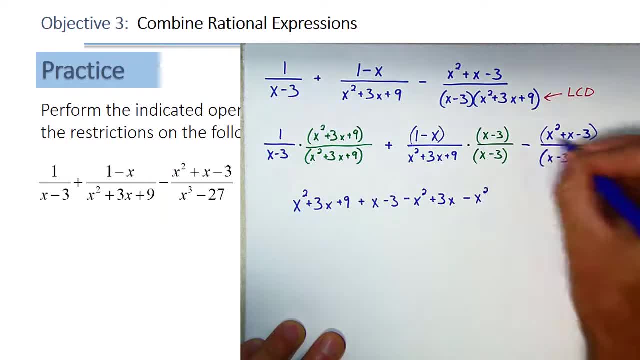 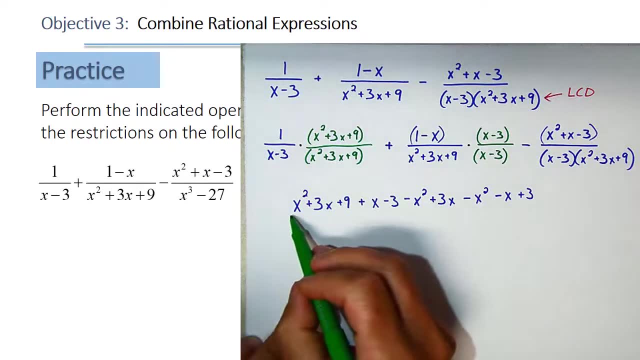 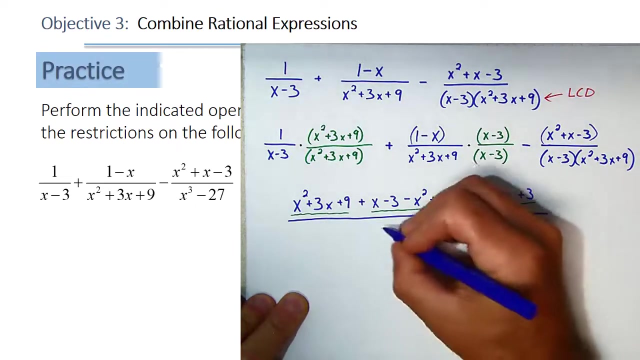 so that becomes minus x, squared minus x And plus 3.. So there's our left numerator, there's the FOIL product of our middle numerator and there's the distribution result of our last numerator. Now, all those are individual terms that are all over our grand common denominator here of 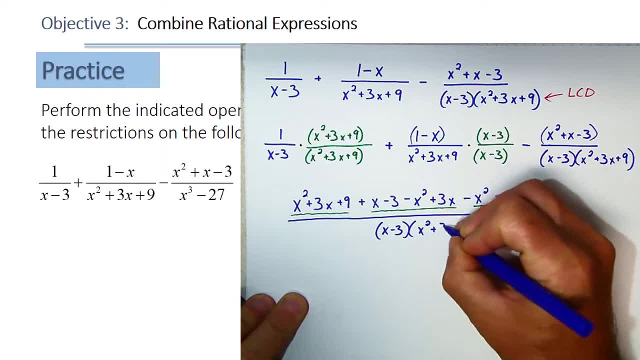 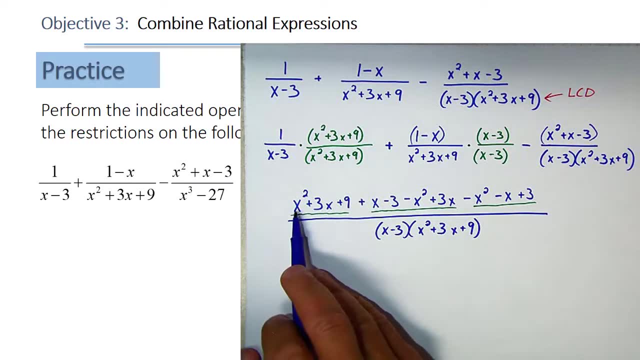 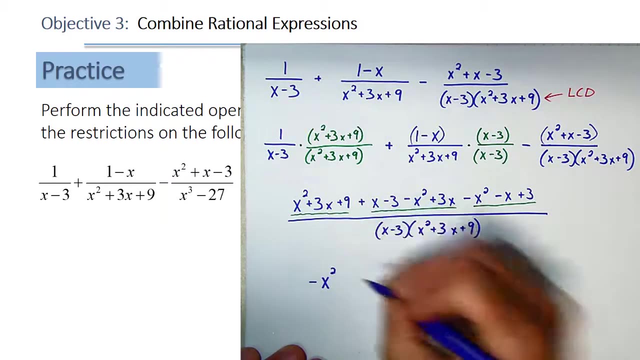 x minus 3 times x squared plus 3x plus 9.. Okay, let's combine all those like terms and see what we get. We can do. we've got x squared minus x squared minus x squared, And so that gives us a total of negative x squared. 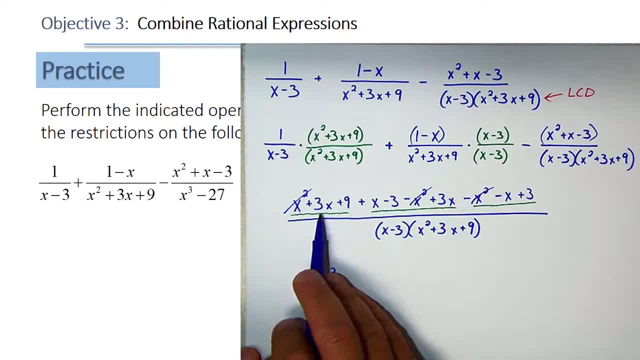 Those are now gone And we have plus 3x plus x. for 4x Plus 3x that's 7x Minus x. that puts us back at plus 6x. And for constants we have 9 minus 3 is 6, plus 3 is plus 9.. 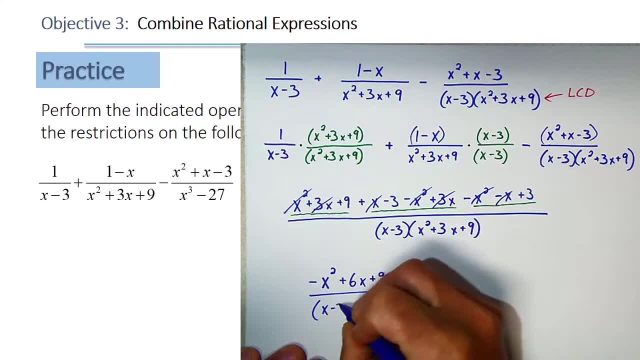 All over our common denominator of x minus 3 times x, squared plus 3x plus 9.. Now can we factor that numerator at all? Well, let's try getting that negative sign out. So if we pull out a negative sign out of the numerator, 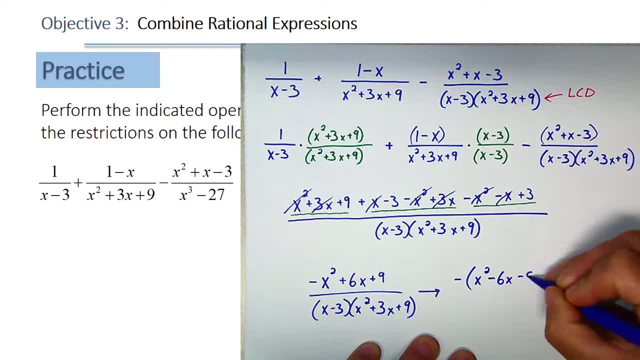 we get x squared minus 6x minus 9. And that sure feels factorable, but it's not, And so we would have to leave that fraction as it is. Nothing cancels, So either one of these two would be as it turns out. 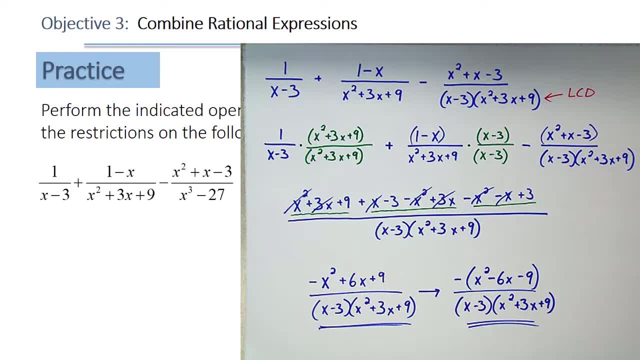 the result of this combining, There's no more simplification to do. Now what about our restrictions? Well, the only real restriction we can deal with here is x minus 3.. Since the x squared plus 3x plus 9 doesn't factor anymore. 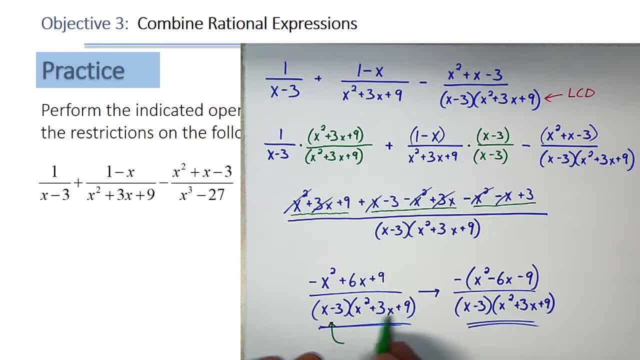 we can't break that up, And so we can't set it equal to 0 and solve As it turns out. that would have imaginary solutions, as we're going to see later, But we can note that x minus 3 is not allowed to be 0.. 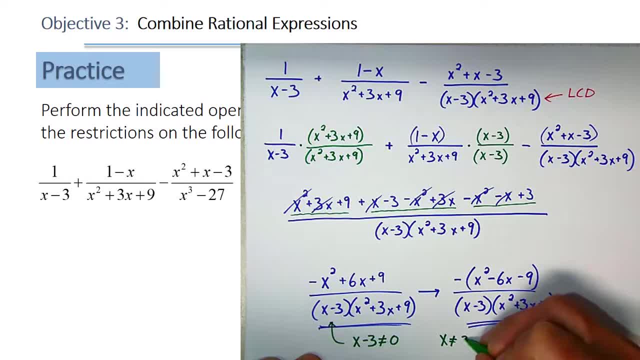 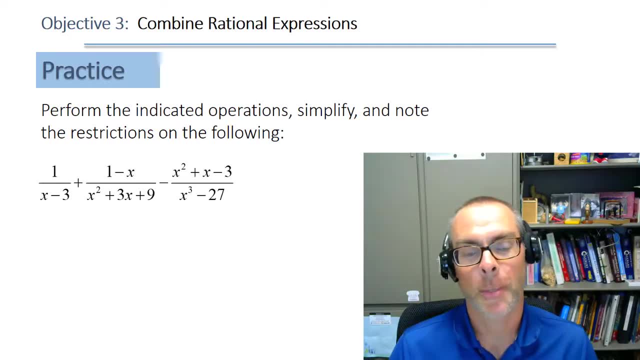 And therefore x cannot be 3.. And that is the one restriction on this expression. OK, Well, before we do anything, I just want to stop. Look at what a messy problem you just worked out Again. your algebra skills are really progressing. 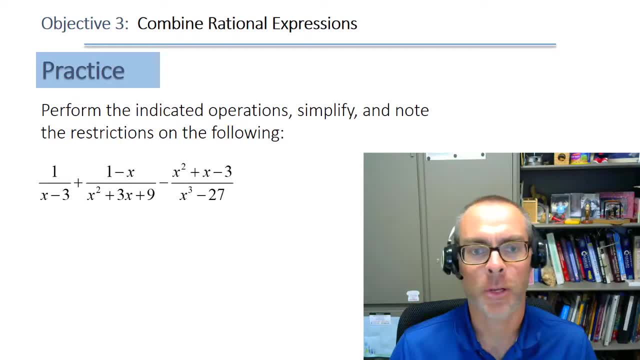 This is a kind of problem where a very, very small sliver of the population would know what to do with that algebraically, And you should feel pretty good. You've got a lot of peaks in here And you're no algebraic lightweight at this point. 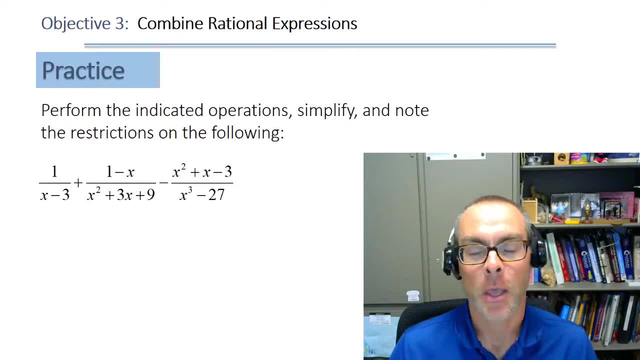 You're doing some pretty heavy duty stuff, So nice job. Keep that up. But that does wrap up this topic With our work. in the previous lesson that taught you how to multiply and divide algebraic fractions. now you can add and subtract them. 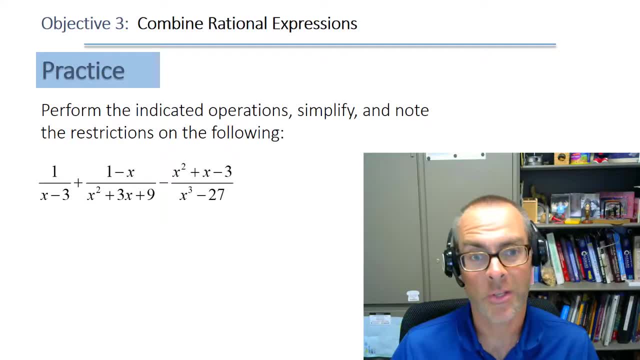 We're well on our way. We're inching our way forward to solving equations that look like this, But we have one more thing to do in the next lesson before we're ready to do that. So go ahead and do the WebAssign work. 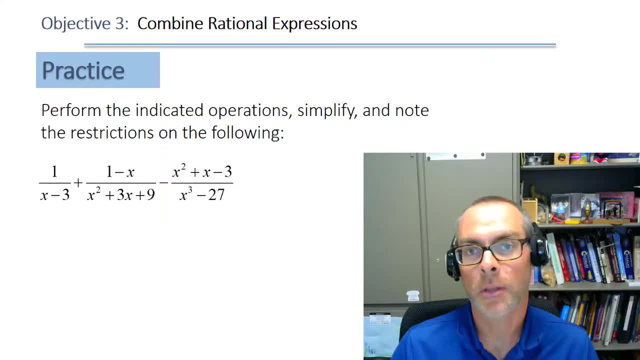 that goes along with this. I'm certainly happy to help you out with anything that comes up. Do an Ask Your Teacher Or, as always, you can set up a little online Zoom with me and I'll work through any of these that give you trouble. Good luck and keep at it.